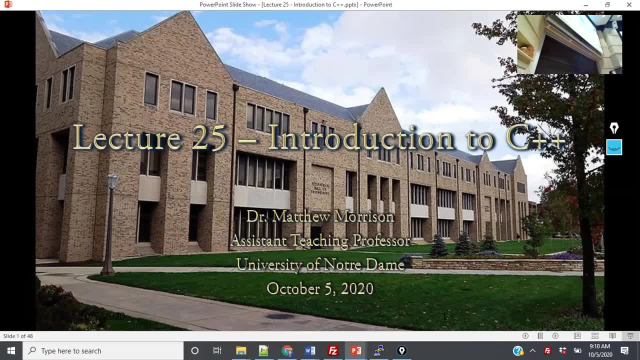 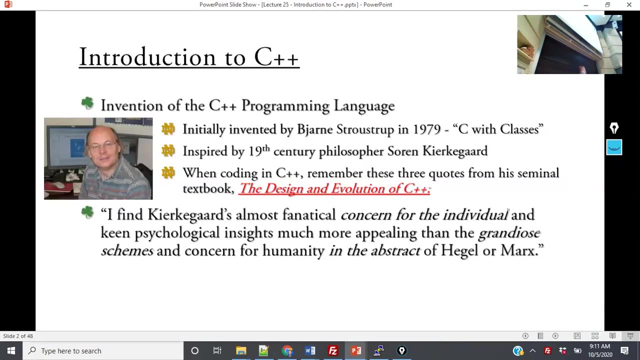 Good morning. So today we are going to switch over to a new programming language. Up to this point, for the first eight weeks, we did seven. So C++ is going to be what we are going to be studying the rest of the semester. And the reason why we want to pick it up here is because the idea behind C++ is building upon what is known as object-oriented programming. Now you had your first kind of brush with objects last week when we were starting to dig into structs. The struct has different private members, well I'm sorry, you see it's public members, but these members could be defined together and put onto the data heap. And so now, it became well, if we can combine things together, are there ways that we can define how they all work together in a more concise way? And how can we make them all work together in a way that aids our computational thinking? So the first thing I want to do before we even dig in to what C++ is and the differences between C++ and C, I want to emphasize the difference between C and C++. 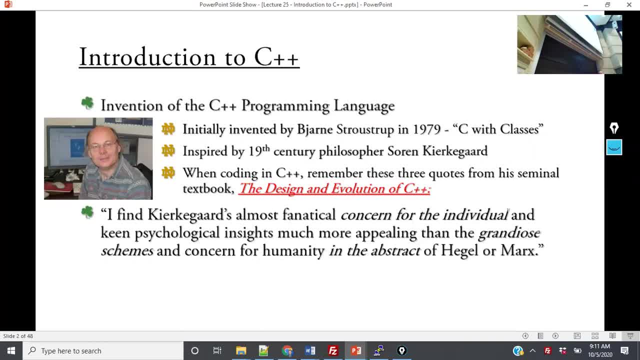 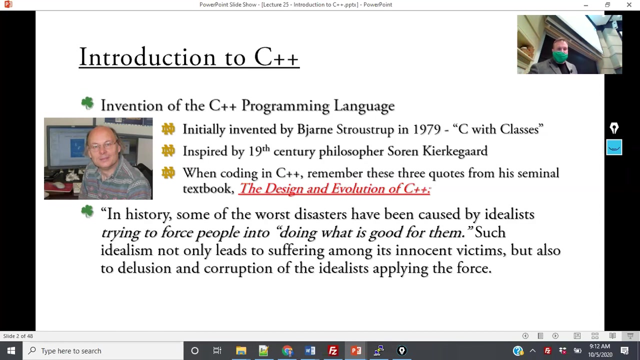 C++ is inherently philosophical difference. And because of this, some of you are going to look at C and C++ in very different ways. So Bjarni Strauss, I have a picture of him here, invents C++ in 1979. At the time he calls it C with classes. And he wasn't inspired by trying to make the program work better, he was inspired by the philosophy of . And he, more importantly why he thought his philosophy was not good. And he has this exact quote here, I find Kierkegaard almost fanatical concern for the individual and keen psychological insights much more appealing, than the grandoy schemes and concern for community in the abstract of Heigl and Marx. And so what he's hitting on here is this idea of trying to force people into quote, doing what is good for them. The idea of trying to force people into quote, doing what is good for them. And then you can't get out of that. 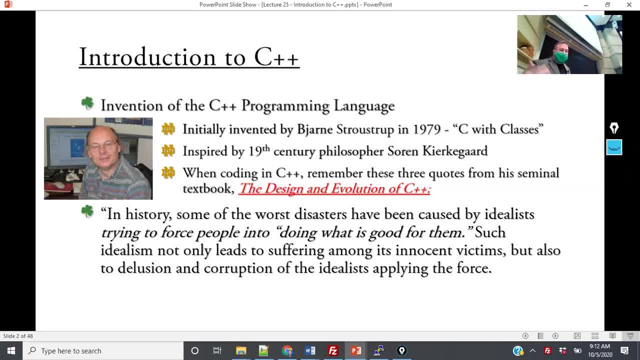 them he says this is the cause of so much suffering in the world and some of you go yeah dr morrison made me suffer a lot in the first few assignments of the semester 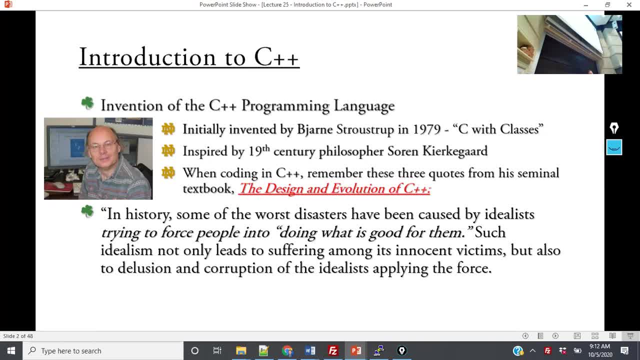 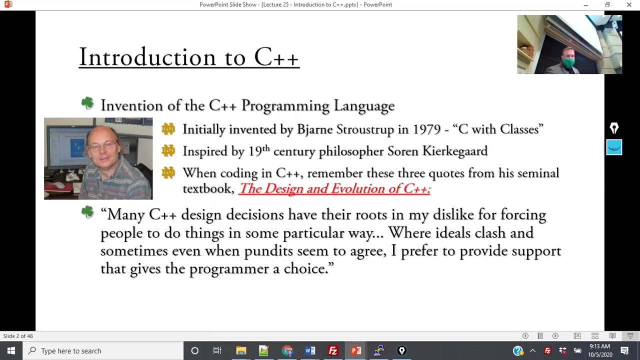 i totally agree with what uh vrna is talking about here but what he's taught what he is specifically talking about is this idea that forcing programming as a purely procedural idea is idealistic and so he creates c plus plus as a way to build upon c in a way that allows them to be able to implement ideas by developing these classes and objects and he says many c plus plus design decisions have their roots in my dislike for forcing people to do things in some particular way where ideals clash and sometimes even pundits seem to agree i prefer you 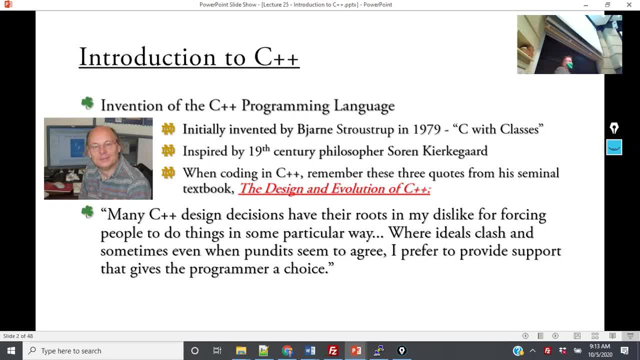 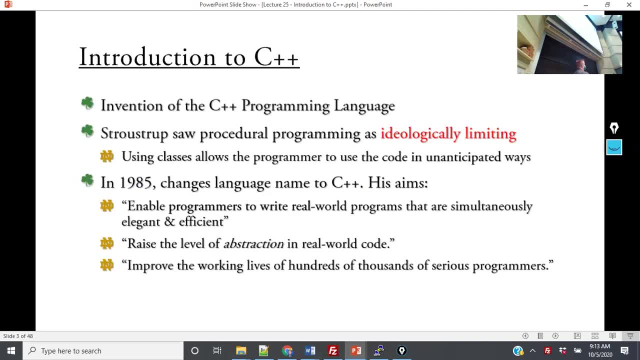 to provide support that gives the programmers a choice so he sees c as ideologically limited and then he tries to build upon this it's an improvement upon c c plus one hence c plus plus and he says what is enables programmers to write real world programs that are simultaneously elegant efficient raise this idea of levels of abstraction so we saw this a little bit when we started writing this book and we saw this a little bit when we started writing the universe of morning and her in me �a's article when she was at the time at supertechnology 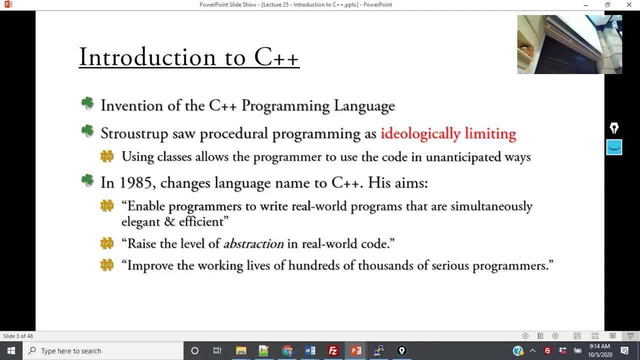 was fledgling by weird characters and they weren't aware that there was also the energy of systems 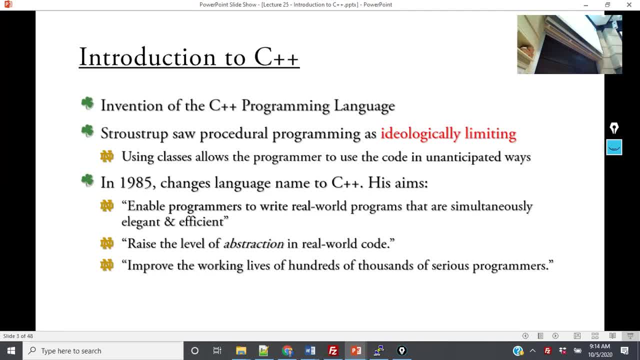 they were in the middle puddle i think i invite a clip of from the middle pub we Triple-A 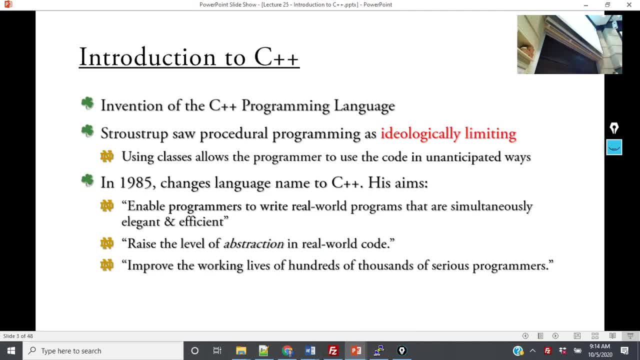 when we started working in structural right so we've had as in the lab that we were working on this week we were bringing in an array of structures that containels a first name a last name and a double for a midterm and a final exam right so when we were using structures you pass the string just passing it by reference by the pole so a lot of this memory allocation that you have to do is starting to be abstracted away from you it's getting a little less complex we're starting to get that margaret hamilton's book down a little bit and so he even says his goal was to improve the working lives of hundreds of thousands of serious programmers in 1985 the idea of hundreds of thousands of programmers as opposed to the millions that we have on earth today was much more realistic so he's trying to aim to make this world a better place for everybody who was programming back then so what is the idea of object-oriented programming 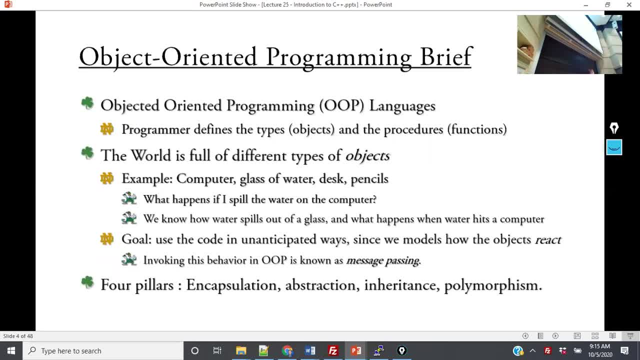 and what the four main concepts that i'm really going to hammer home for the rest of the semester are encapsulation abstraction inheritance 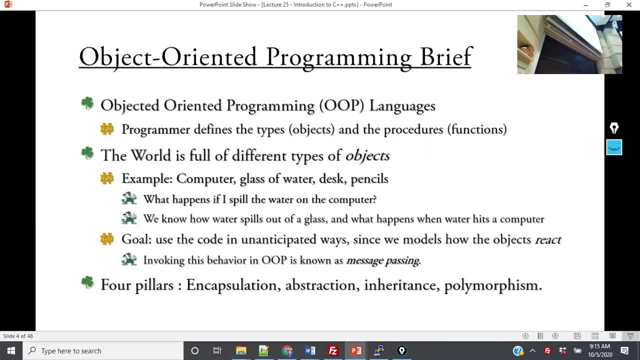 and polymorphism i'm going to define all of these into this lecture 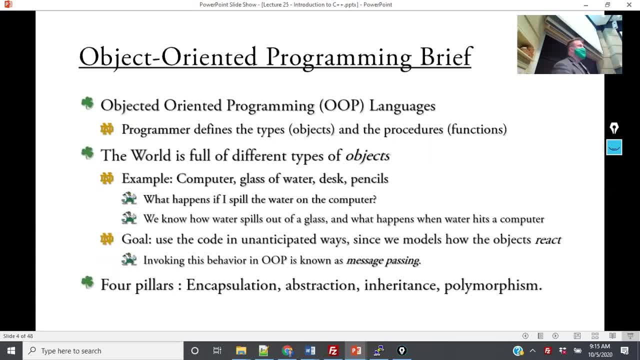 but first in order to understand all these we have to kind of think about what the world is like not what the program is like so the world is full of objects you know for example i'm holding 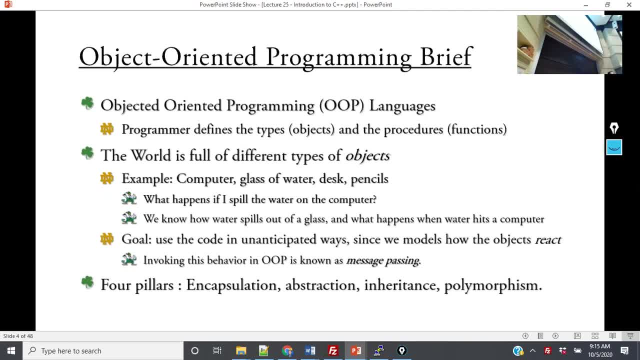 disinfectant right and if i were to unscrew this disinfectant and spill it all over right there are several things that would happen when i would do this i think i would do this i have to account for gravity i have to account for how fast things go i have to account for what's in the bottle and then i have to account for what will happen when the disinfectant hits the desk 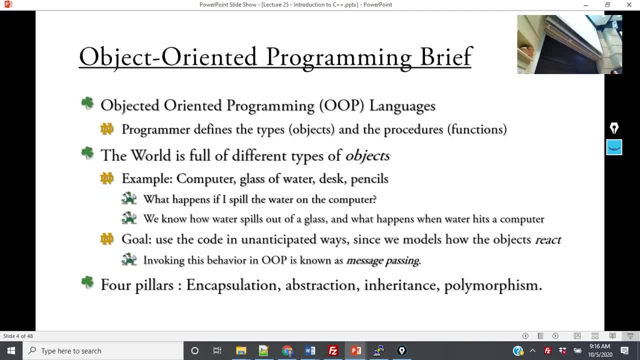 so there are certain things that can splash if this wasn't disinfected this is some sort of other chemical material that were to actually spill in here i could potentially create some burns it could potentially create some bad odors we'd all have to evacuate the room there's a lot of things we have read about where this could happen because all kinds of different things that can happen based on one of the contents of this bottle so it's not just okay right function turn over bottle right function splash 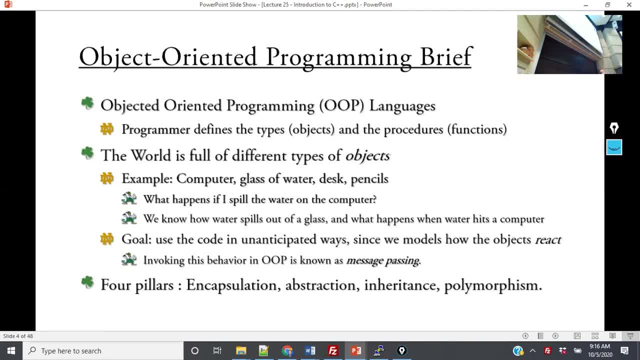 it's not possible to account for every possible thing with C++ the objective is to be able to make objects work together such that when we have unintended interaction 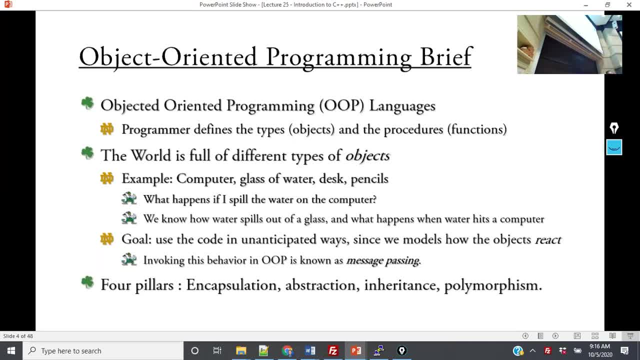 we can predict it as best as possible through the objectsubject to during the plant interaction and ultimately you'rehmmm 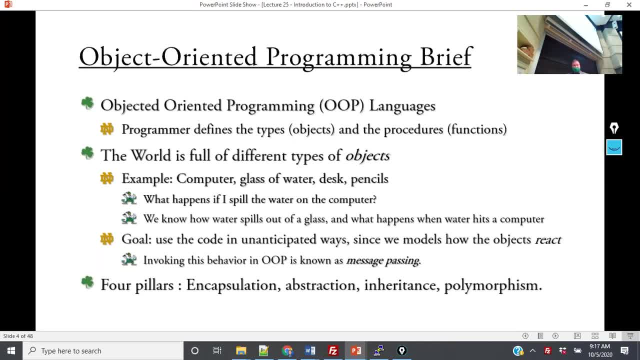 operations so on this slide what i have is an example of a glass of water a desk and some pencils if i spill the water on the computer it can potentially damage the computer but it's not we don't have a function when glass tipped over break a break computer right what we have in this object are if i tip the glass over what's going to happen if i have water hit the computer what's going to happen and when those two things combine they should work seamlessly with the goal here of making the program work properly when it's used in unanticipated ways 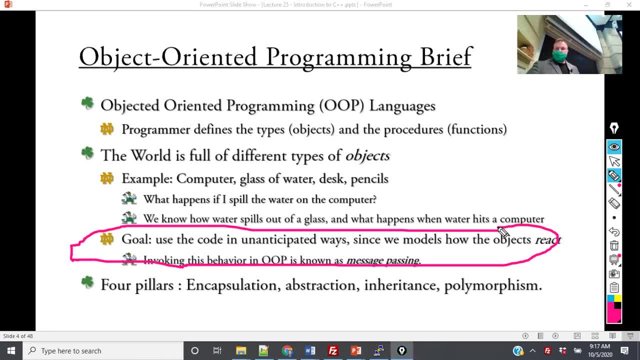 and we're going to hit on this idea of message passing message passing is us passing information back and forth between objects and classes 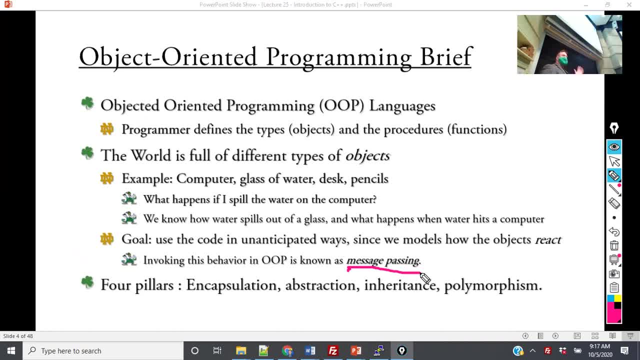 all right so just everybody have a general understanding of what i'm trying to get at for the moment 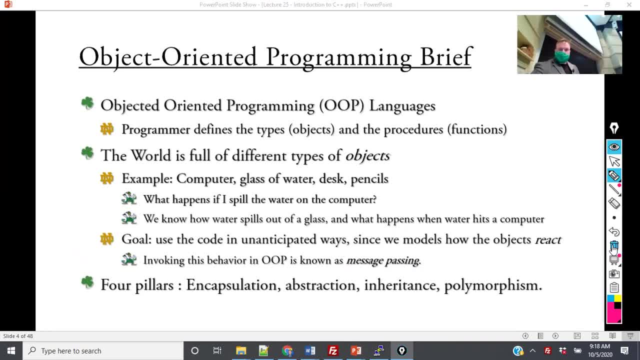 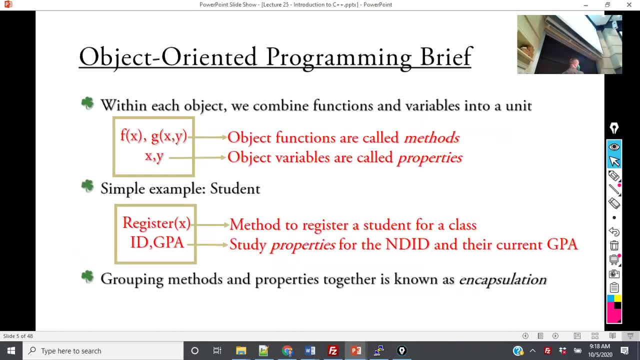 all right so how are we going to break these classes down and how do we think about these ideas 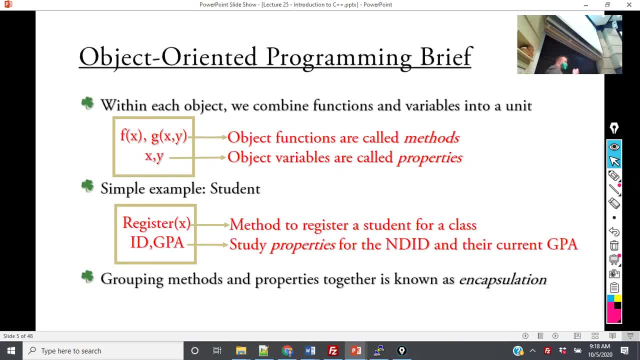 so first when we have so what we've learned about in structures this idea of properties or members 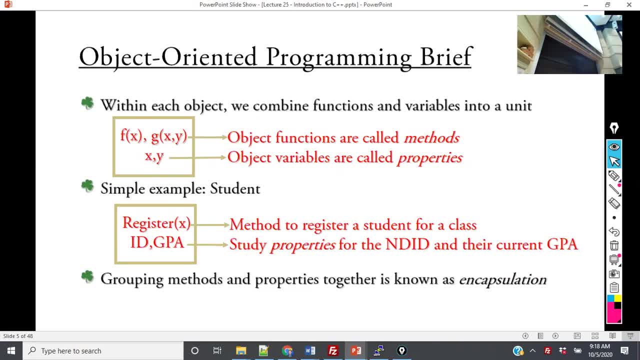 or objects or a specific object or objects are 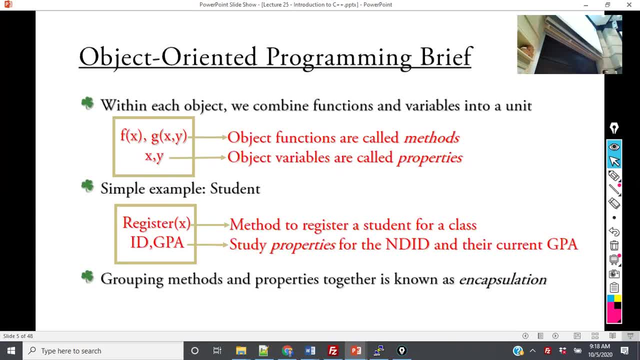 you things you can use to define a specific object for example i have this water bottle it has several different properties it has color it has weight it has a volume it can contain it has a name on it electronics cleaner and disinfectant zeph right all of these things again a warning label for external use of finals okay let's just set it on fire um there's all kinds of things that i can add as members or properties of that object but the new thing that we are going to discuss here is this 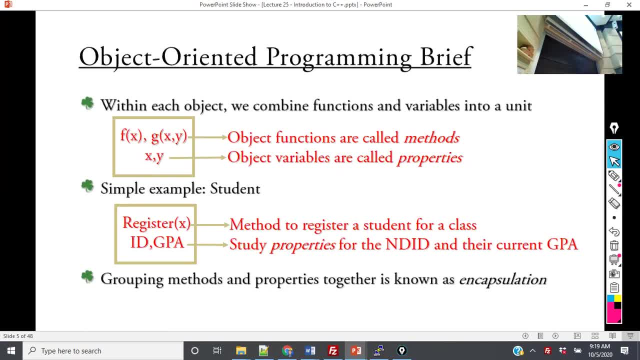 idea of methods methods are going to be functions within a class that are acted upon when we call a class object so for example when we had that structure right when you had to calculate it you had to access calculate the final average you had to access the two members bring them out in another function and perform the result right what if we could write a function calculate final that is a method of that student and that all you have to do for the programmer is say 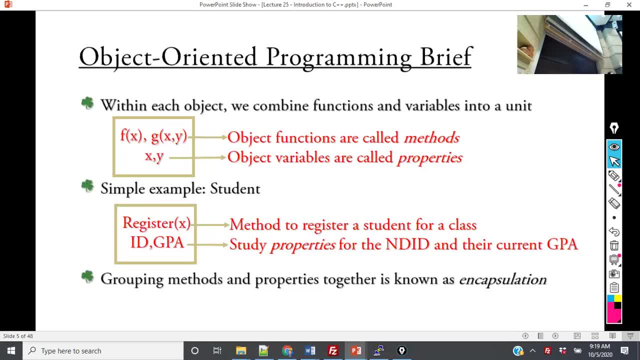 what's their final average you call final average function would be student i dot final average and then it just returns it for you automatically this is what's known as a method we're going to see several examples of this later in the semester so i have two examples here of a simple example of a student where it has members or properties 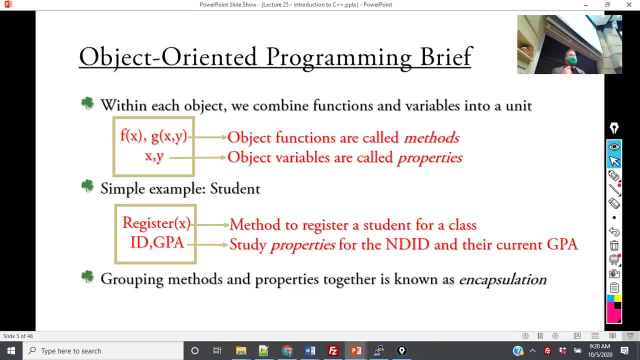 their student id their gpa and then i have a method register so i want to register for classes it's a function that would dictate to the student how to read an information and then based on that student's information we can determine whether or not that student should be allowed to register for specific classes 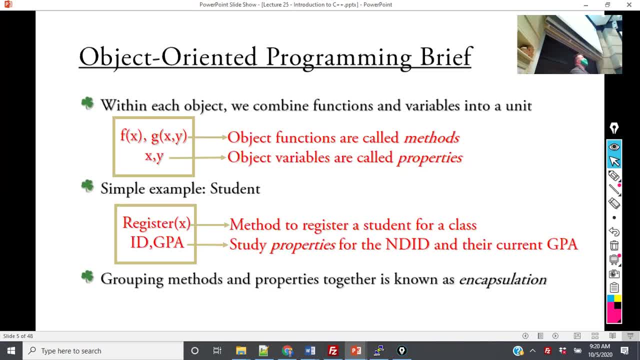 and putting these all together inside of a class whether it's the operations that can be done on the data and the data that's used to define the object 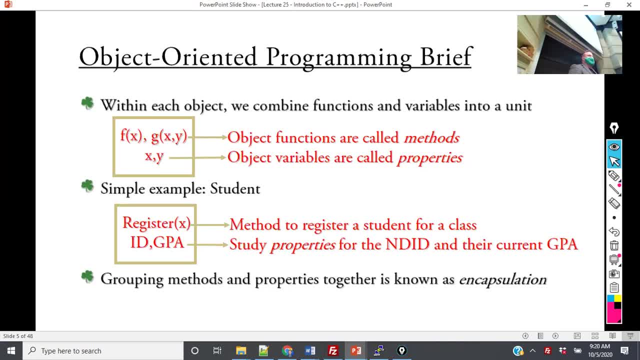 putting them all together in a class is known as encapsulation so we're just encapsulating every thing kind of in its own bubble right so grouping methods and properties together is known as encapsulation all right if you have any questions before we continue let me quickly check the chat 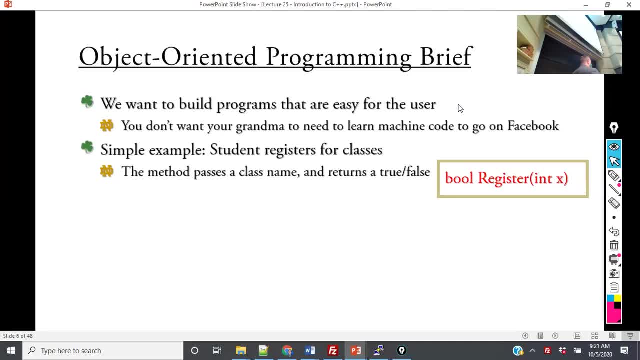 next so some of you are most of you are probably are sophomores some of you are juniors some of you are seniors so registration is different for each of you some of you are allowed to register on a certain day some of you have to wait until a different day some of you have a certain number of credits some of you have certain other restrictions 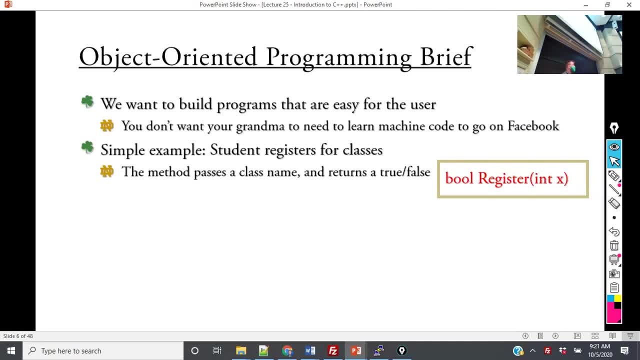 now for example maybe you're doing whenever if we're ever allowed to leave america again you get to go into london for angie london right you have all these different things that are restrictions based on who the type of state and this is where it comes down to our experience and student you are so it's not just enough to define an object we have to be able to come up with ways to be able to say that we want students to be able to do a certain thing so for example in this register function i might have a private function called prerequisites i pass a certain information within the student and it does some work for me and then it's returned publicly in the register 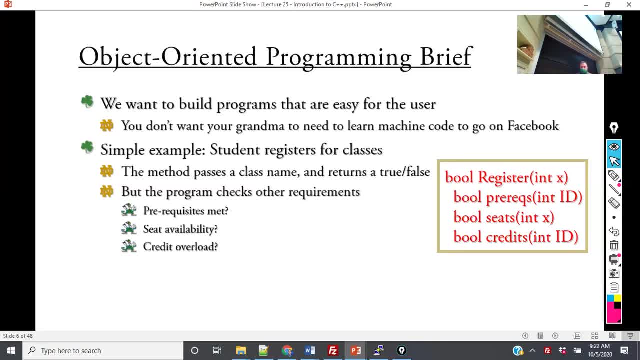 method so we can define methods inside of a class to break things down modularity inside the class 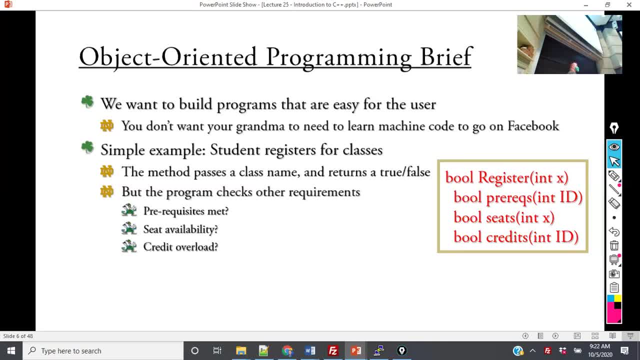 that can be reused within the class but cannot be accessed publicly by the programmer and this is good we want to you 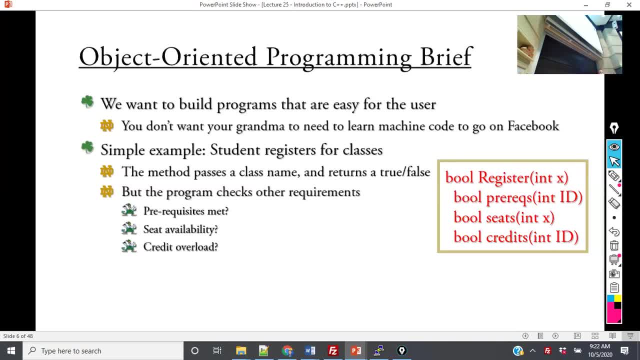 remove a lot of the complexity away from the program for example when you write f scan f right you write an f scan f function you pass everything by reference and then some magic happened right you didn't need to know what was going on and then it would return and everything would work 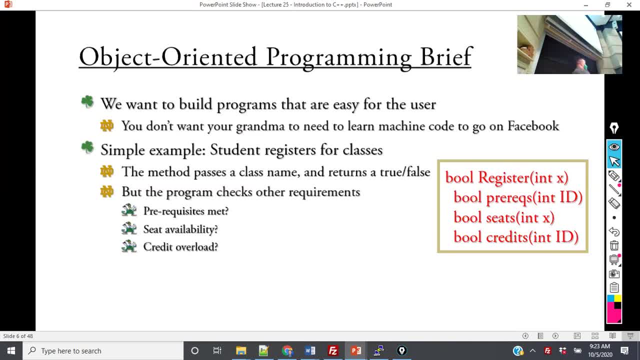 this is the same thing in c++ you one of the programming paradigms is that you want to hide some of the complexity away from the programmer and hiding procedural complexity away from the programmer is known as abstraction 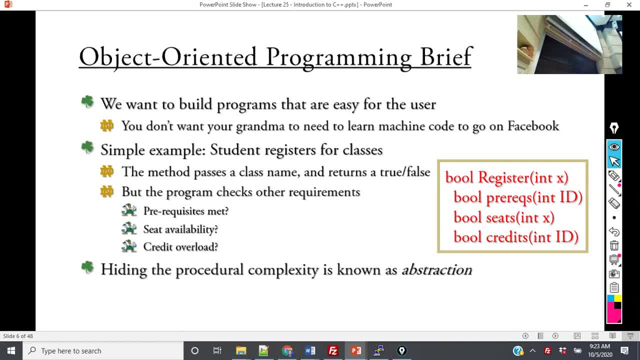 if somebody is using your program and they only need to write you write three or four lines of code and it does everything they wanted to do they're going to love your code right oh wow i was able to just call this function that did all this other stuff i didn't need to write it so that's one of the things about object oriented programming is you want to be able to draw from there regardless of the function that's used or not if there's an Scikit-learn 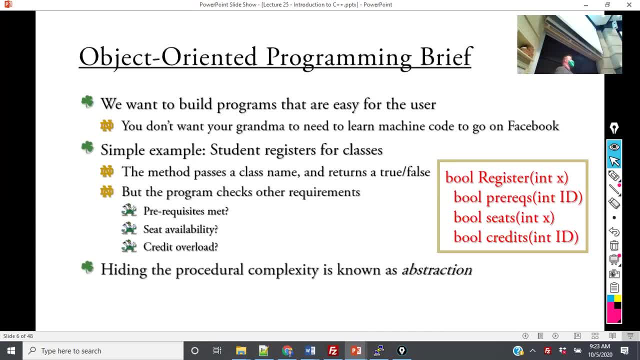 want to only have the user write what it is that they need to do in order to complete the task, and then you can allow the abstraction in the object to do a lot of the work for you. 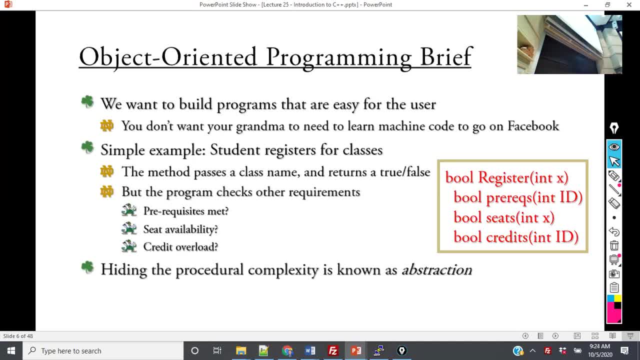 So, for example, let's say that I'm acting like an idiot, and I ignored this warning, right? I have mashed, and I have my formable liquid, and I put them together, and it ignites, right? 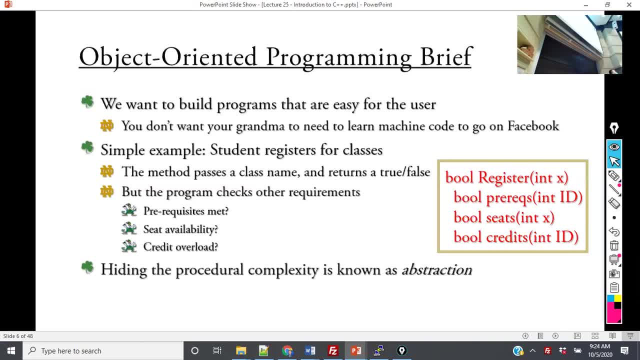 The programmer doesn't need to calculate all the chemical equations that are going on underneath in order to determine whether or not it's going to ignite. We have, we can have a private method that allows us to be able to form those calculations, and then we could return on fire. 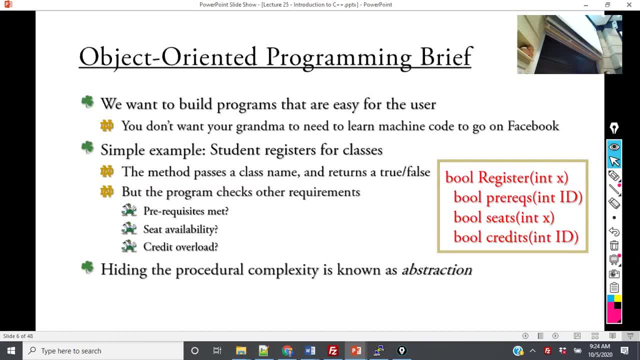 That abstracts the complexity away from the programmer. So, this is a big paradigm in object-oriented programming. 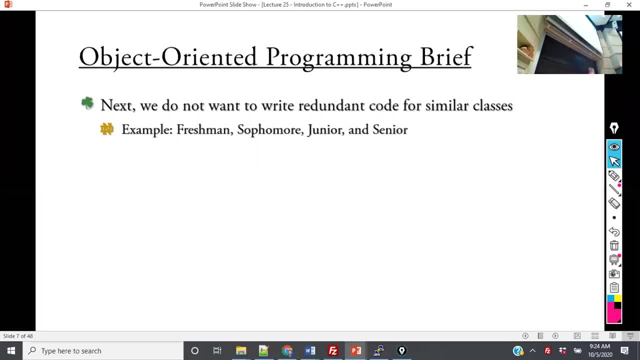 Next thing, because many of you are sophomores, many of you are juniors, many of you are seniors, you want to do the same task, but in a different way, which means we don't want to have to read, write redundant code for similar classes. 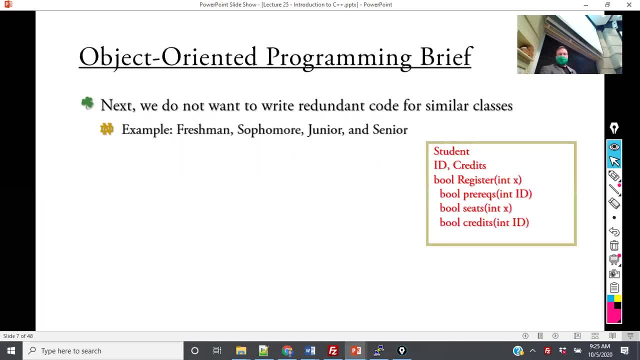 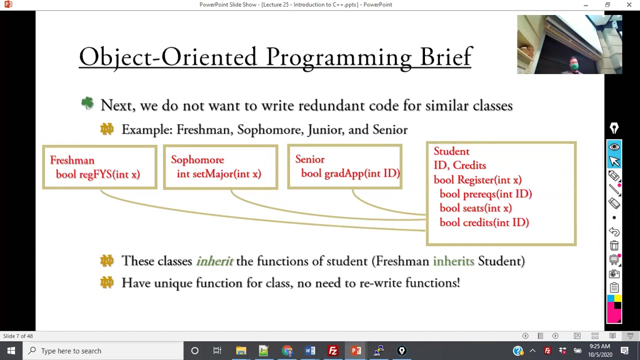 So, a sophomore, for example, so, I'm sorry, for a student, you all have registers, you have information for ID, you all have information to keep track of the number of credits you've completed, and so on. However, for freshmen, you have some sort of registration function that indicates you have to do stuff for the first year of studies. For sophomores, you want to set your major. Come up with some way to indicate that you are setting your major, and this is something that doesn't need to be done for juniors or seniors in the event, you know, you're not setting your major the first time. You can change your major, which is a different function method entirely, and then with seniors, you have a function to apply for graduation. Now, imagine many of you sophomores want to do that now, but unfortunately, we can't let you. So, these classes and methods, we can define them to be unique to each object type. 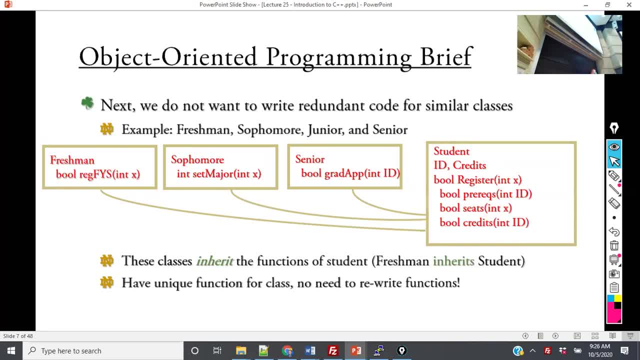 So, we can say that a senior is a Notre Dame student, and therefore, a senior should have some basic fundamental things that are similar. So, we have things that are similar, sophomores, juniors, and seniors that they all have in common, and we can define a base class to have all that information, and then the derived classes will inherit those fundamental things. We call that process of writing multiple classes inheritance. You see here that these classes inherit the functions of the student, that a freshman inherits that basic information, and then what this allows us to do is it allows us to be able to write unique functions for freshmen, for sophomores, for juniors, and the benefit is that we will not have to rewrite these particular methods. So, this is one of the things that we should think about, not just in terms of coding, but in terms of computational thinking in order to be able to describe the world. 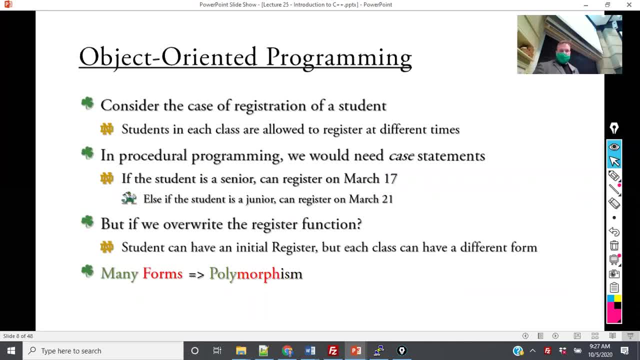 So, here I have considered the case of a registration of a student. 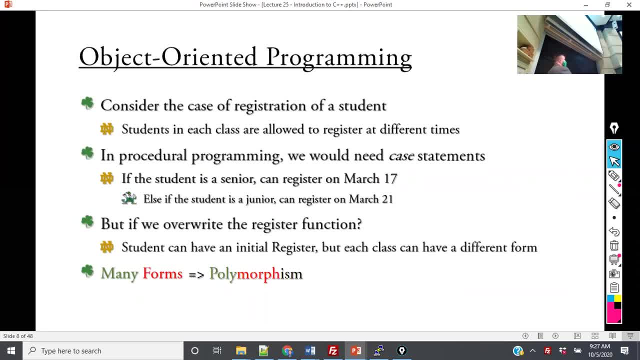 We have in procedural programming, we would need an insane number of case statements in order to do this, right? If a student is a senior, can register on March 17th, otherwise a junior, March 21st. Sophomore, March 25th, and so on. But, what if in each class, these derived classes, I just write its own version? That is, in register, if you're a sophomore, you can do this. Register, if you're a junior, you can do this, and we can separate it out in an object-oriented manner. Furthermore, I don't want to have to write a method, register sophomore, register junior, register senior. All of these things are in order to do this. 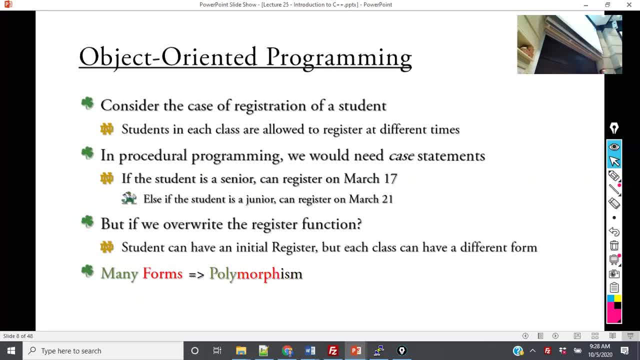 All we're doing is we're registering. But underneath, we can abstract that complexity away. 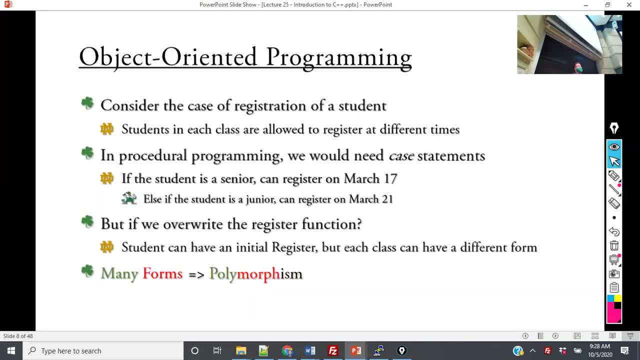 If we rewrite the name of the same function in that new class, in that derived class, we can create another form of it. We're rewriting it. 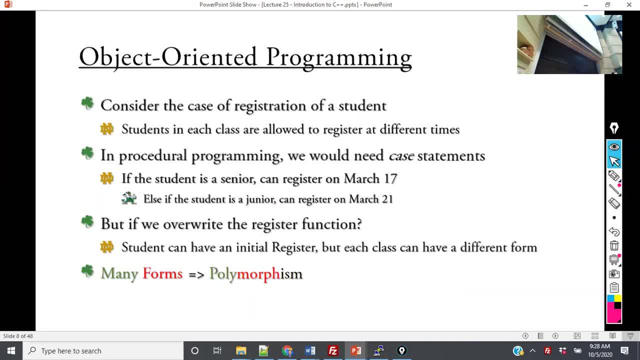 So, these functions across these different derived classes can have many forms. If you go into Greek, that's polymorphism. So, that is our fourth term. 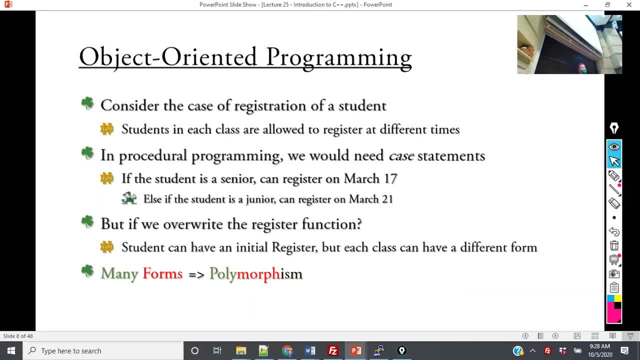 So, the fundamentals, encapsulation, be able to come up with ways we're going to use this idea of classes to describe ideas, fundamental ideas, and we will encapsulate them together. Second, with object-oriented programming, we want a programmer who is using our code to be able to implement this as efficiently as possible without having to do a lot of the back-end work. 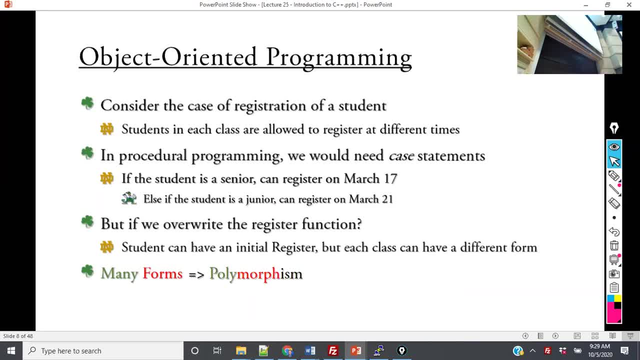 So, we want to abstract the complexity away. The third one, we want to think about ideas as a base set of ideas and derived ideas. For example, student versus freshman, sophomore, junior, senior. And that, at first, all of these should have a base idea. In order, they're related in ideas. There should be things that they have in common. And that the derived ideas should enhance them. Those base ideas. And then, fourth, we have to think about these different ideas can have the same type of task, but have variations on the task based on their properties. 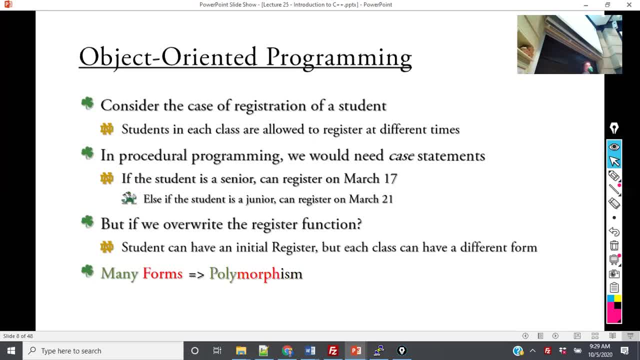 So, we would have many forms of this task, which is polymorphism. 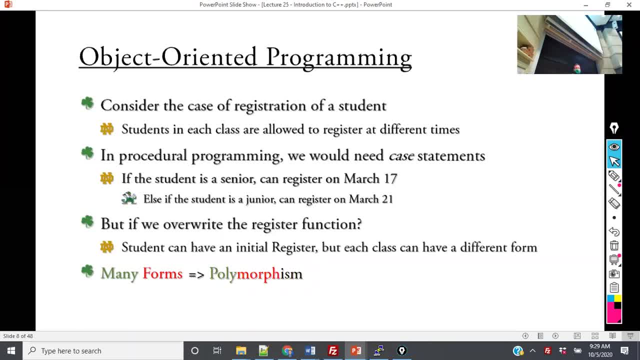 Does anybody have any questions on this before I continue? Let me check the chat. Same thing. Okay. 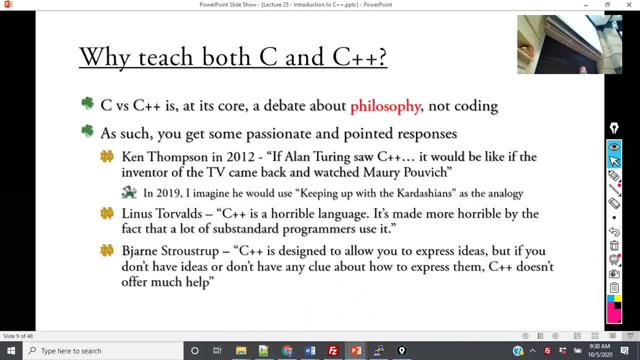 So, trying to come up with wild and crazy ideas like building off of procedural and coming up with object-oriented programming, as anybody who's trying to change things in the world can tell you, doesn't always go over that terribly well. And, you know, when you're attacking the people who do the previous thing, they tend to not like that. So, Ken Thompson. 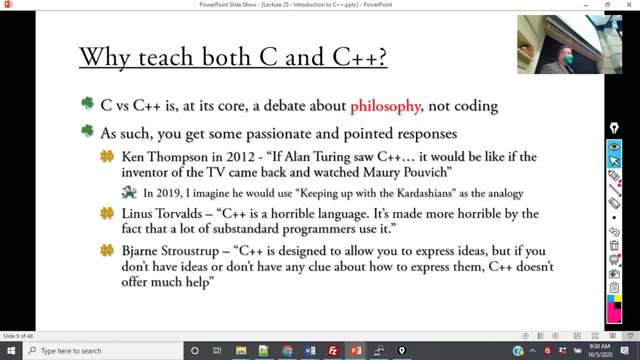 He responds to this idea of C++. Ken Thompson is one of the co-inventors of C. And he said, if Alan Turing saw C++, it would be like if the inventor of the TV came back and saw Maury Povich on the television. 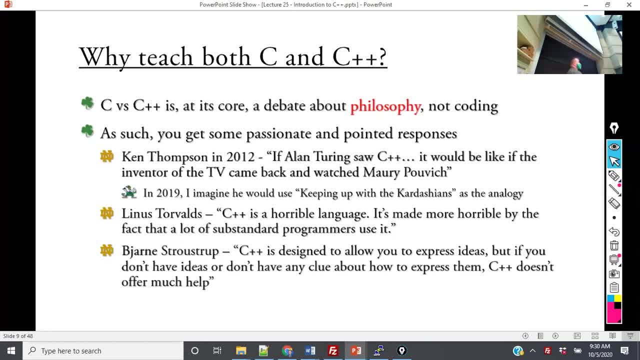 So, pick your least favorite TV show. That's what he means, right? 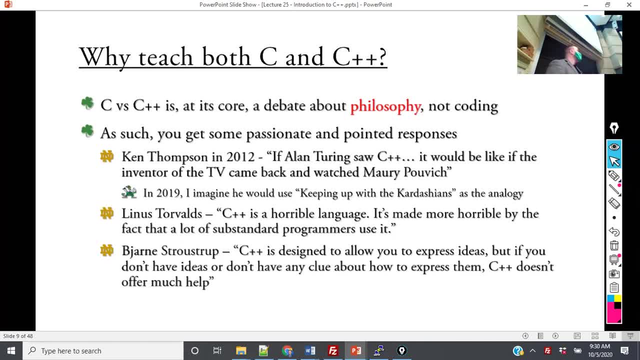 You're one of those people who doesn't like keeping up with the Kardashians. That's a good one. You know, like USC football. That's another one. Whatever it is. 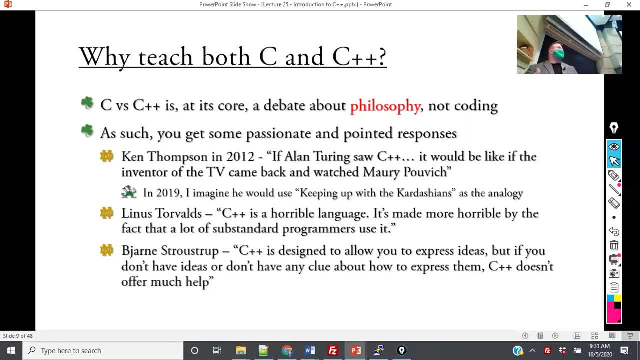 So, he said, Alan Turing invented the computer, and he would see C++ and go, oh, my God, why did you put that on that machine? Didn't like it very much. 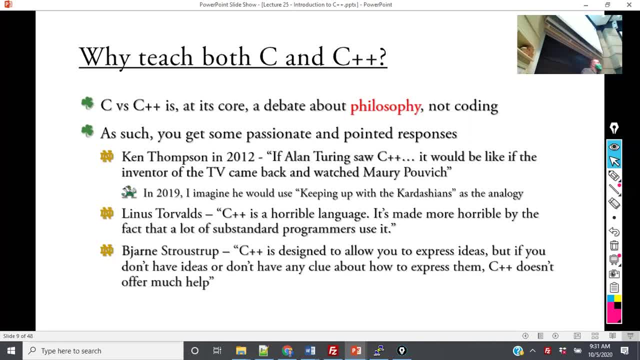 Linus Torvalds, the inventor of Linux, which we program on when we use the Notre Dame machines. He just straight up, C++ is a horrible language. It is made more horrible by the fact that a lot of substandard programmers use it. So, then, Bjarne, he responds and says, C++. It says, C++ is designed to allow you to express ideas. But if you don't have any ideas or have any clue how to express them, then C++ doesn't offer much help. 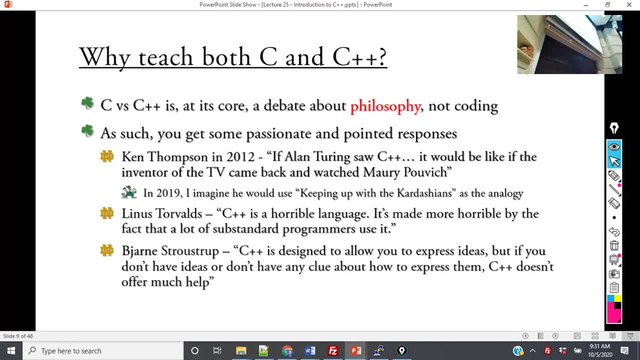 So, it's a lot of shade going on here. 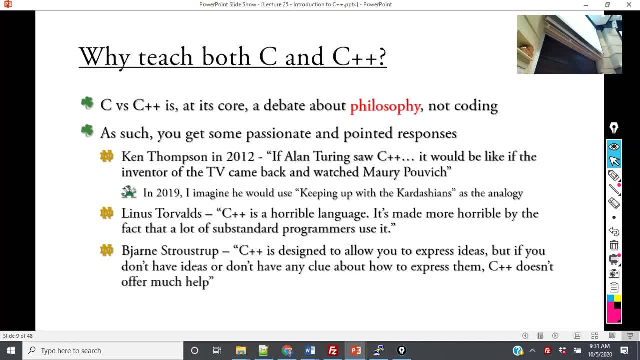 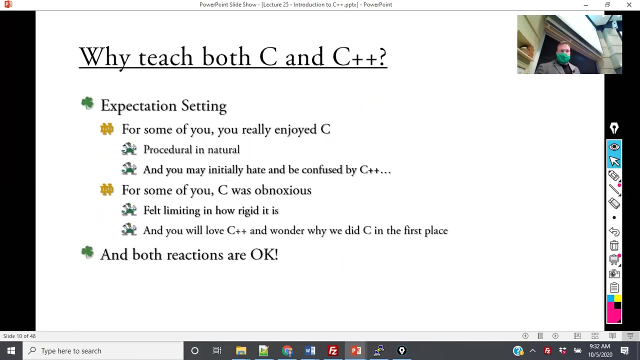 The difference between C and C++ is not just programming. It's philosophical. It's kind of the same way if you look at different actual languages. You know, you're trying to convey an idea in French. Versus trying to convey an idea in English. Versus trying to convey it in German. It can come off in very different ways, right? So, C and C++ can be very similar. 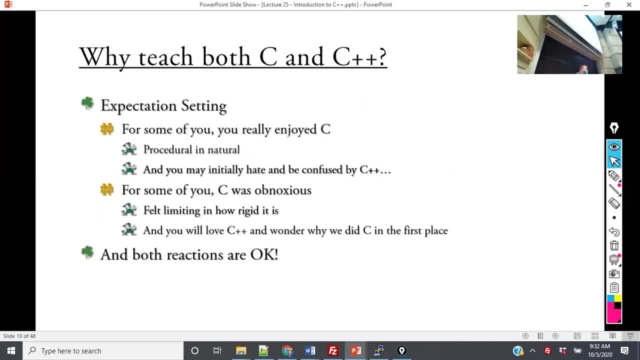 And so, why do I tell you all this? So, it's important to do some expectation setting as we transfer from C to C++. 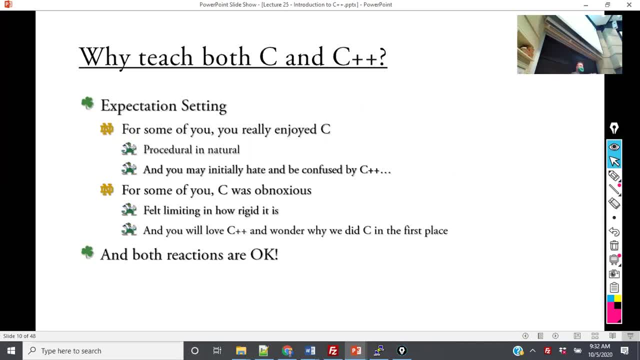 For some of you who really enjoy programming in C, you know, it does it in a very specific way. And I like being told to do things in a very specific way. Transferring to C++ can be kind of frustrating. Because it's a different kind of thinking. 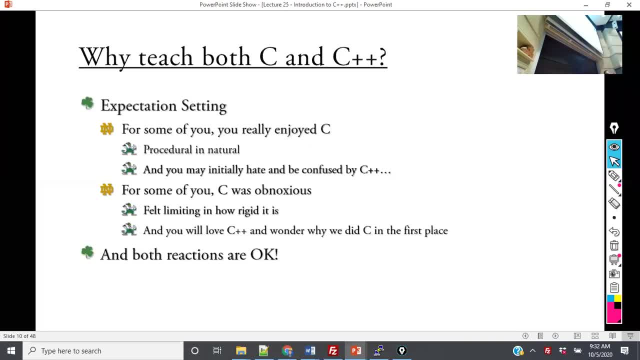 Likewise, some of you might say, C++, I feel it's very limiting. I do this thing. It does the result. 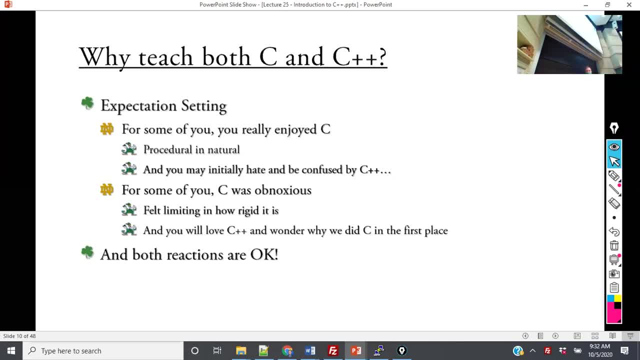 But when I do it, I do really cool stuff. And you will enjoy C++. 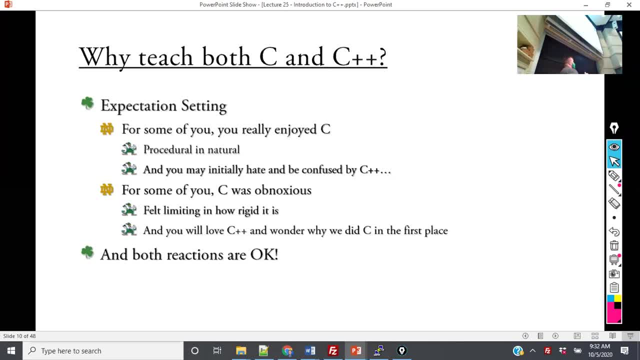 Because C++ kind of goes into that type of thinking. And both of those reactions are okay. It's perfectly fine. 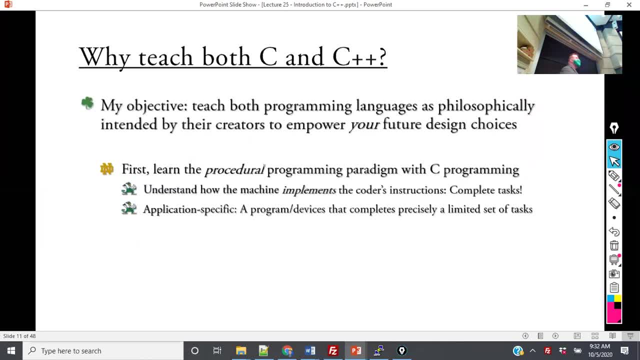 So, the question is, why teach both? The reason why is empowerment of choice. At some point, when you make a decision about what programming languages you're going to use, you want to keep track of several things. The amount of memory it's using. 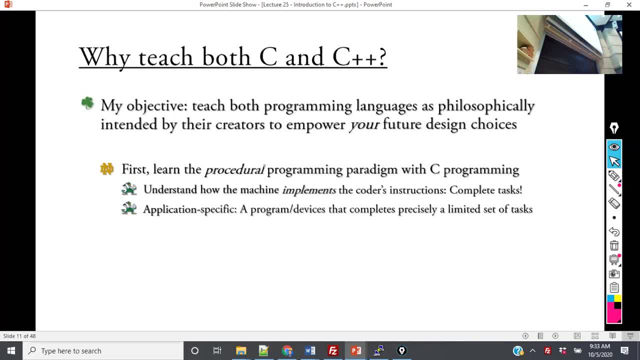 The efficiency of the programming language. And if it's trying to do what it is you need to do. 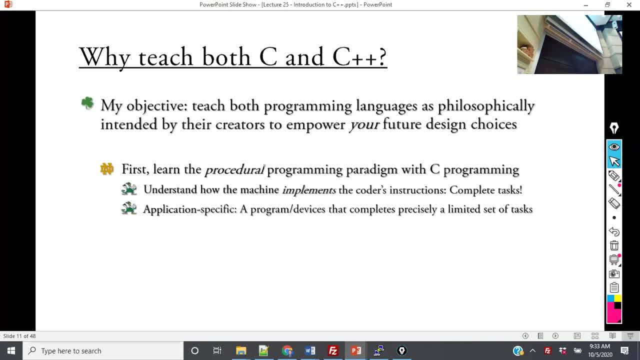 So, a lot of programming languages that have really extensive libraries. For example, Python is a good example. Java is another really good example. Those extensive libraries. Those extensive libraries come with design costs. If you've ever run Java on the Java virtual machine, sometimes you can work really slowly. Because there's a lot of overhead in order to abstract that complexity away. 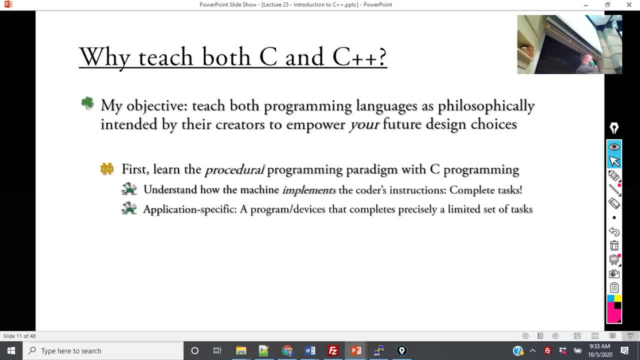 With C and C++, they're both much closer to the actual machine. So, in C, we went to a lot of detail about pointers and how it works to be able to implement things on a certain device. And this is the idea of procedural programming. So, now that you understand how the machine works, now you understand what's going on underneath the hood. Which is going to make what you're understanding of the object-oriented programming significantly better. Because, if you just try to implement the object-oriented programming without an understanding of how the pointers work and how everything's going on in computer architecture, they can really struggle with that. I'll share another Bjarne Strzok quote with you. He said, the thing about C, if you're bad at programming in C, you'll die a thousand times. But, if you're bad at programming in C++, you could potentially blow your mind off. 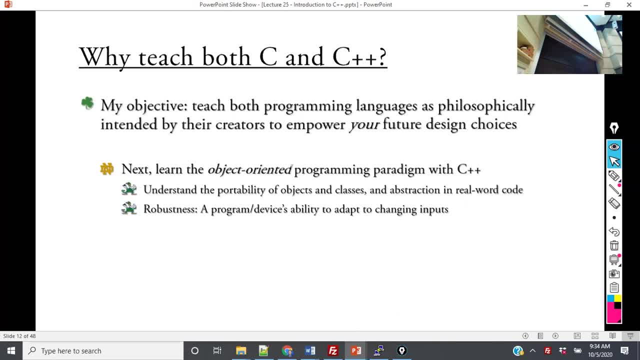 So, there's all kinds of ways where C++ and object-oriented programming can go very wrong for you. 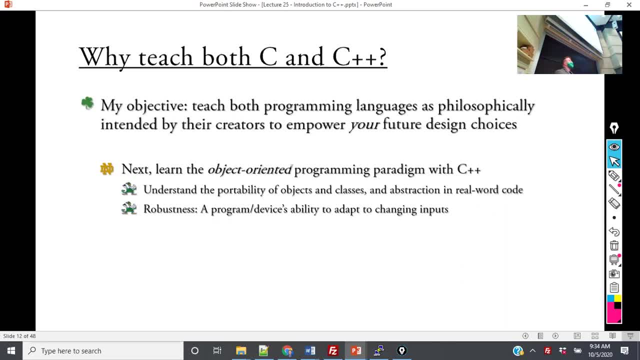 However, if you understand what's going on procedurally, then you're less likely to run into that challenge. The other crucial thing is robustness. 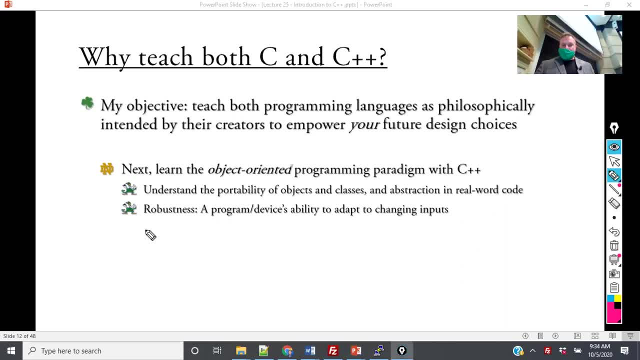 Can we make our program work with as many possible things as possible? So, if I'll create an array and a data structure that we're going to learn about in this semester. 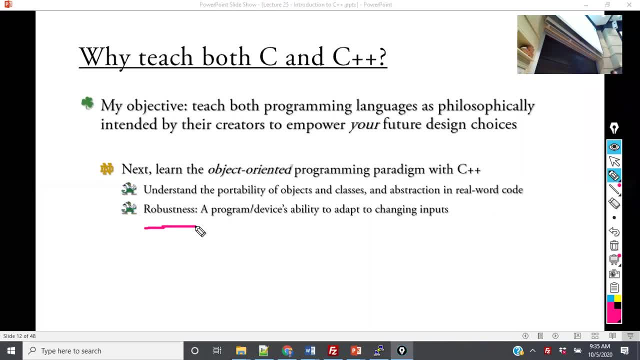 We have what's known as a standard template library. C++ has what's known as a dynamic array. Which is also known as a vector. Which can change the amount of memory that you have allocated to an array. 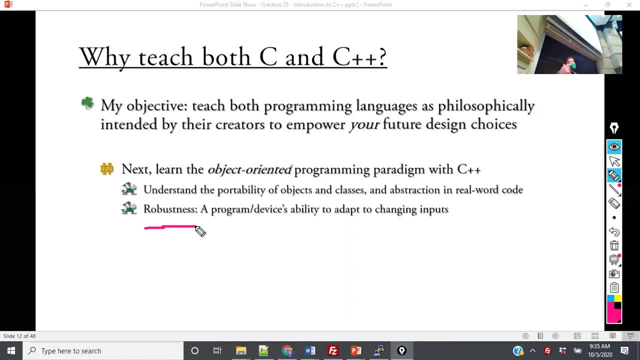 As you start adding in more information. How does it do that? 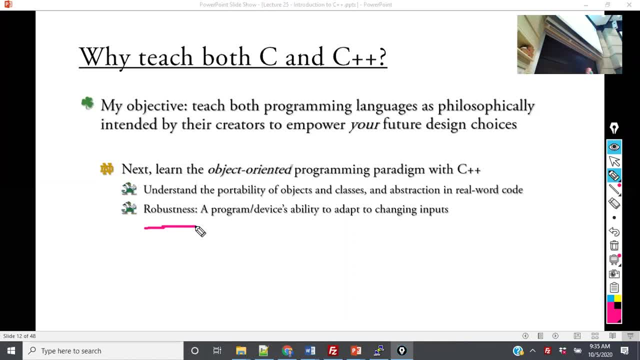 It extracts the complexity away from it. You keep putting them in there. And then some magic happens. And then you're still able to access that information. Just like it's a normal array. And everyone is happy. 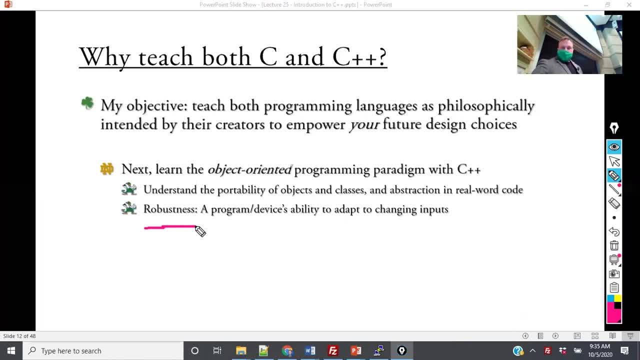 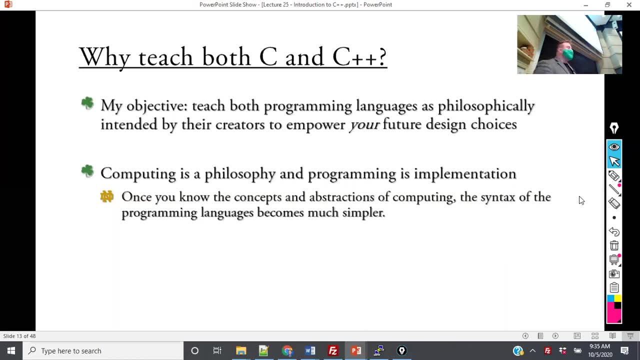 Right? So, ultimately. 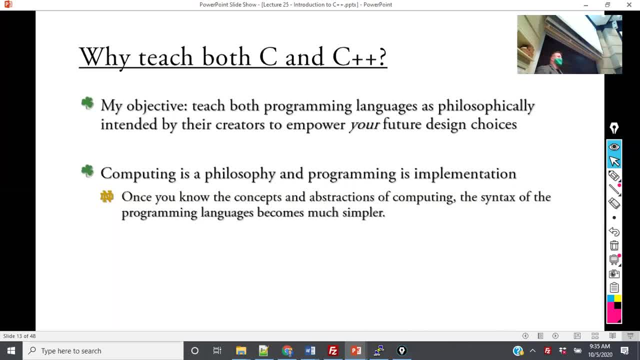 Computing is a philosophy. And programming is an implementation of that philosophy. As you're starting to work on more and more of these assignments. And you're starting to, you know, in familiarity with different programming languages. Getting code in and done in systems. Maybe you're familiar with Python. Maybe you're familiar with Java. You're eventually going to develop your own philosophy of programming. And that's ultimately what introduction to computing and this idea of computational thinking draws down to. 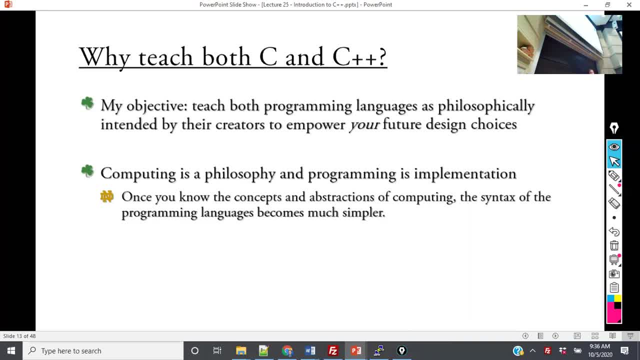 You have the empowerment of choice. To determine which programming language you should use for a task. Which ones you are the most comfortable with. And how it is that you want to accomplish your goals. Skip over that. Okay. 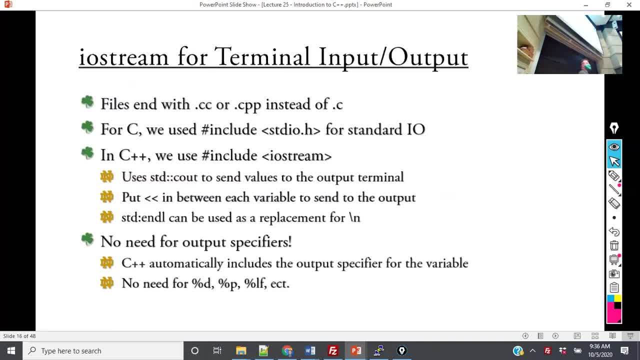 So, does anybody have any questions before I actually start digging into what it is that C++ actually is? Let me check the chat as well. Okay. 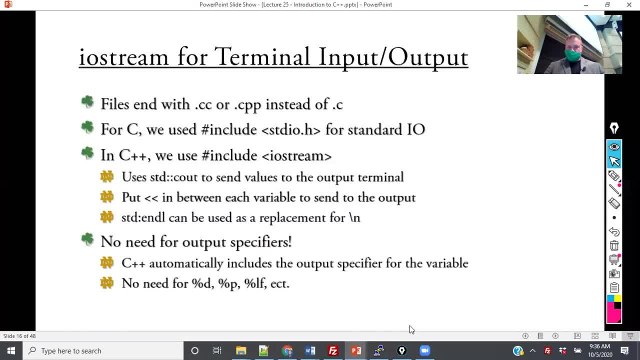 So. So, let's go all the way back to Hello World. So, C++ is Hello World. It's a little different in C. 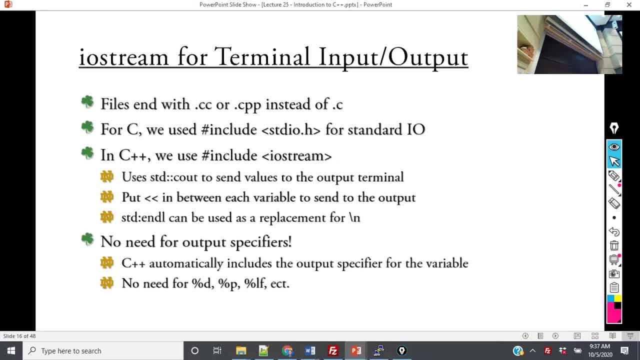 First, in C, they have a library called standardio.h. Right? 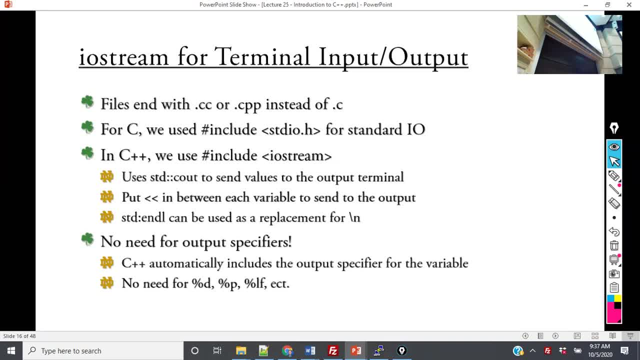 And when we learned about building our own libraries, we used .h files to store that information. And we're still going to do the same thing in C++. 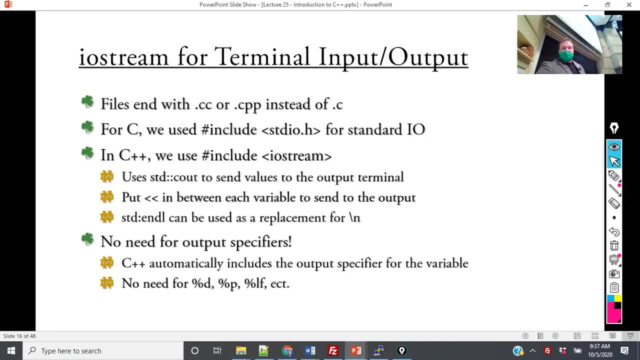 Except when we include libraries, you're going to find that most of them don't have a .h at the end. 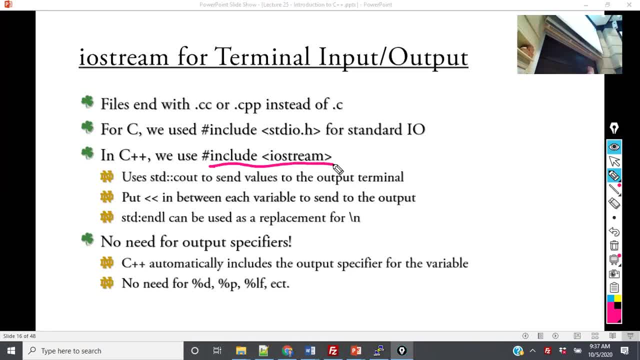 So, the first thing we're going to do is we are going to use iostream as our first library. Input, output, stream. Like stdio.h is standardio. Now, standardio stream. Can be much more robust. In terms of including libraries for us to be able to read in and output information. And we're going to use, instead of fprintf, our output stream is going to be called cout. And we're going to use standard cout. To be able to read information to the output. 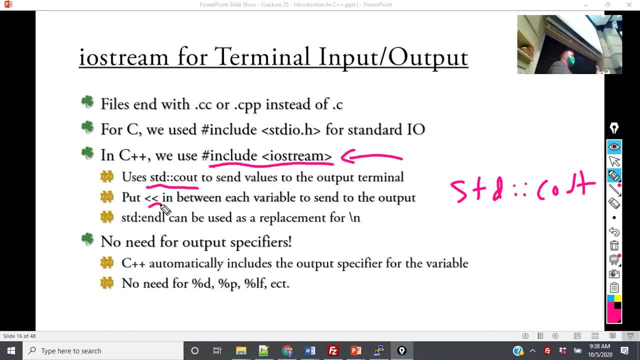 And then what's going to happen is. We're going to be able to put variables and objects in a line to output how we want them. 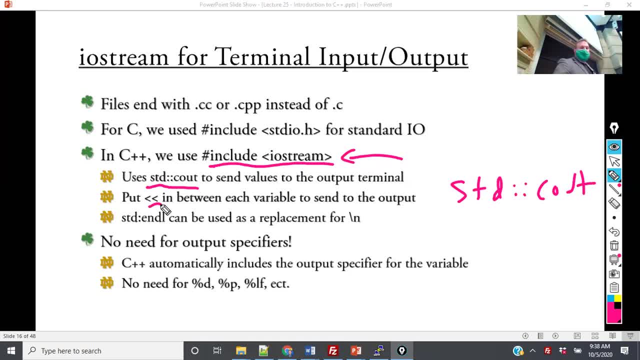 So, this eliminates the need for output specifiers. So, no more of this %t, %p, %lf. None of that. 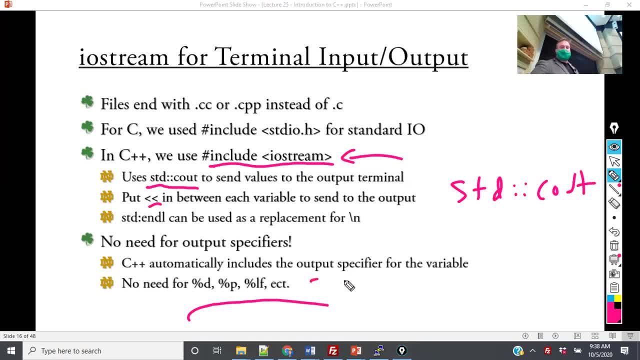 What this is going to do is it's going to automatically include the output specifier for the variable for you. So, we're already seeing a simple example of abstraction. In c, we had to dictate using fprintf. 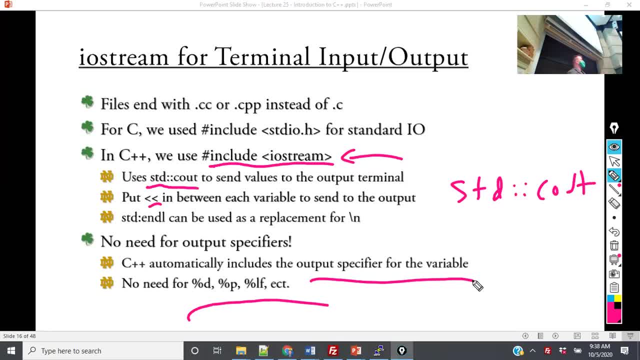 The precise number of characters we need to allocate on the data theme. Which we would then print out. 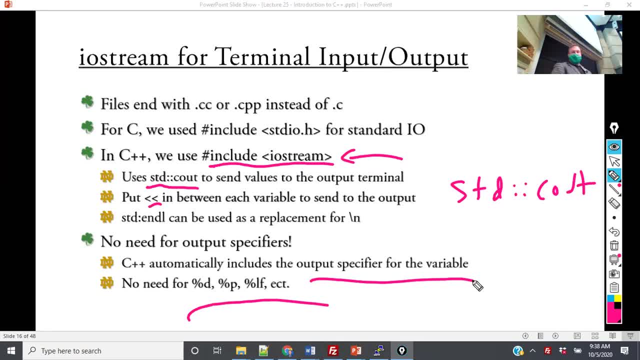 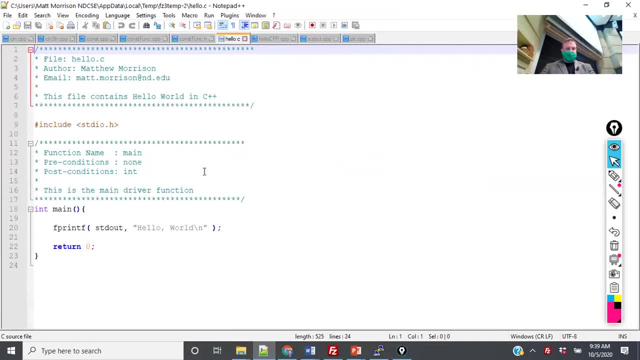 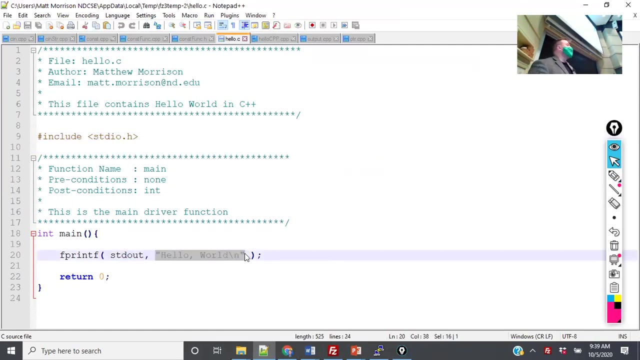 C++ is going to abstract a lot of this complexity away for us. So, let me show you. First, I'm going to review and show you hello.c. So, we remember from hello.c. All the way back to standard io.h. And we had this standard out. We went through and we put all these characters. I have this back. 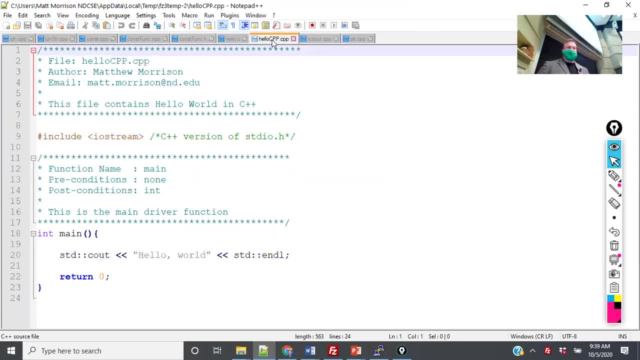 Slash n. In hello.cpp. Instead of using standard io. We're using iostream. And then we have standard out. And then we have hello world. And then we have this end line. Standard end line. Endl. 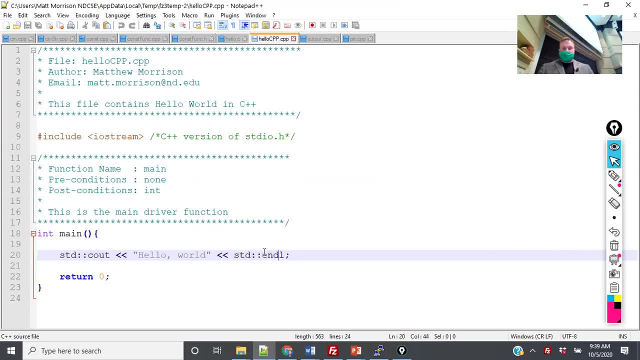 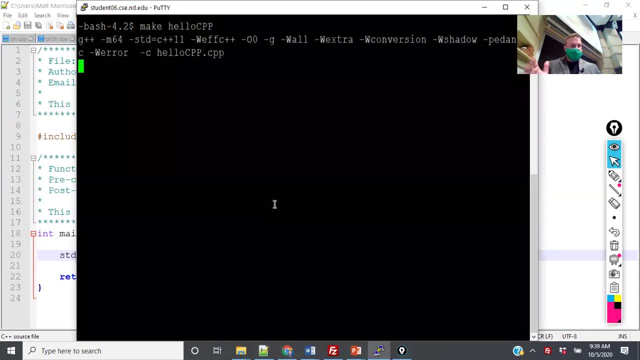 So, first what I'm going to do is I'm going to just run a compilation. Make hello.cpp. And then run it. And it just prints out the same thing as we've done before. 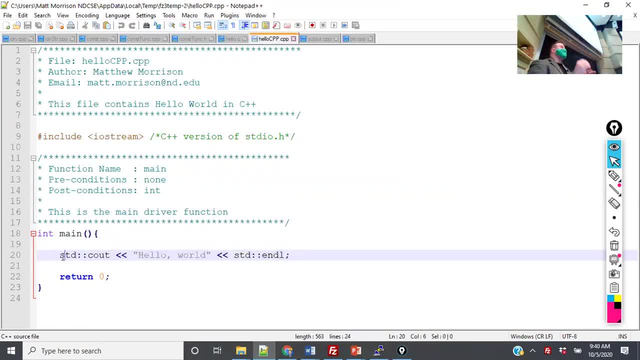 But, now instead of having to constantly do output specifiers, it's a little easier to modify. So, if I say hello world. And then I were to do another space here. Right? Actually, even better. 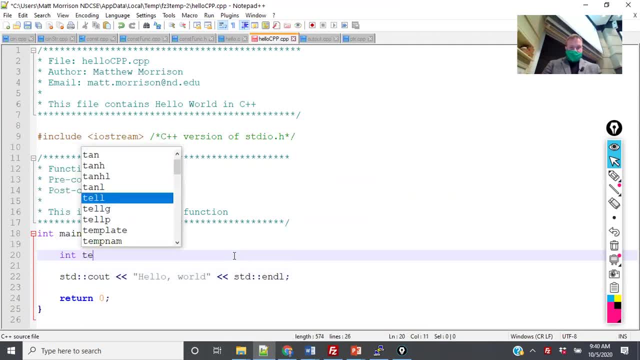 I'll just say int temp is equal to five. Right? 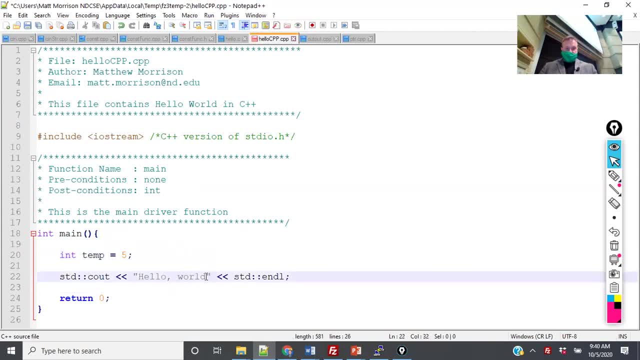 And if I say hello world and put a space. And then I just put temp here. Like so. Does everybody see that? 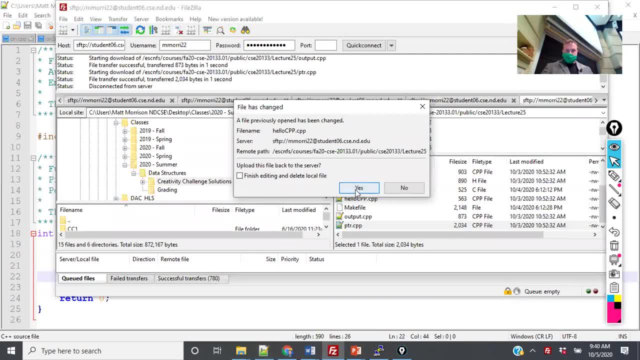 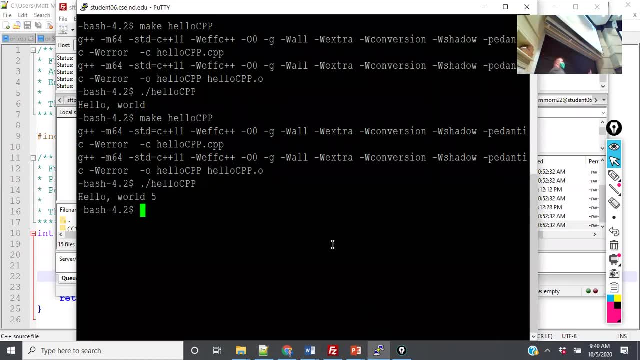 When I print this out, it's going to say hello world five. So, it has abstracted its output specifiers away from us. We have been able to put two different objects of which the iostream has interpreted as a string and an int for it. Does everybody see that? Yes. Yes. So, the follow-up question is does. 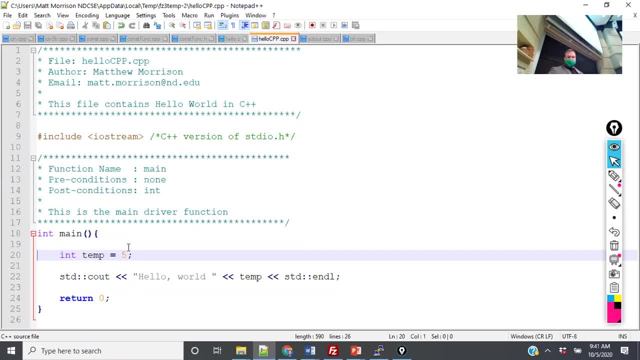 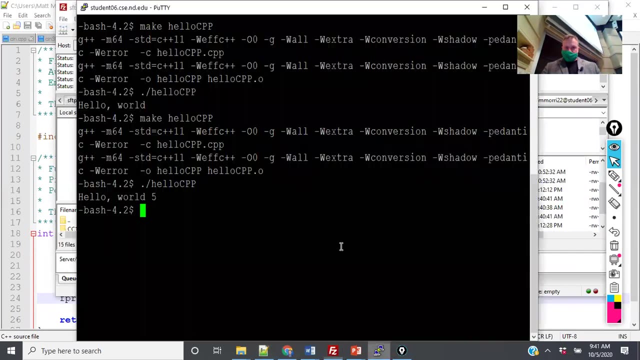 So, C++ is a superset of C. So, I could actually do this. I could actually do fprintf, standard out, hello again. And let's see what happens. 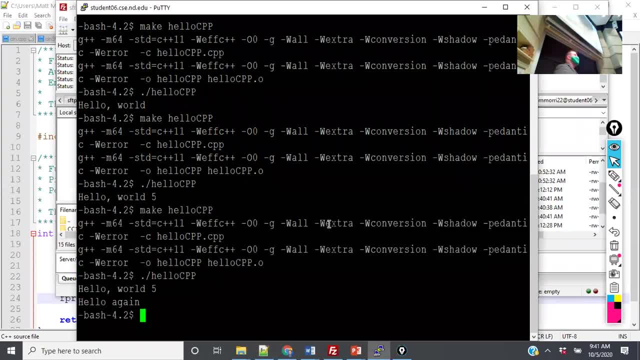 Let's see. We do not. 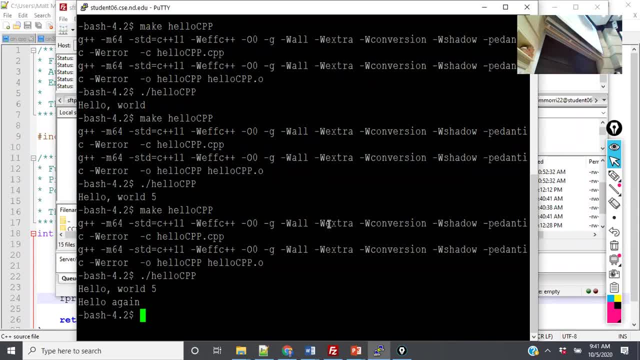 And the reason why is because the iostream is a superset of the library of standard i and i. So, you can do both. 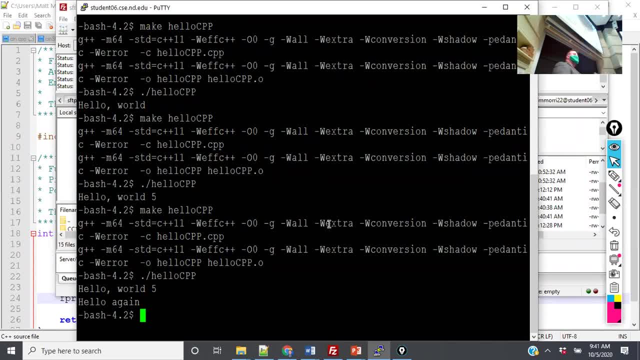 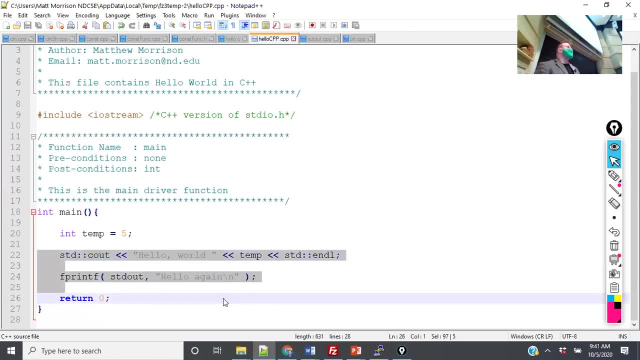 And so, the question is, to kind of go further, when would I want to do both? So, the thing that, as with everything in life, and particularly in programming, there's pros and cons. So, the pro of this is that the more variables I add, it's a lot easier. Right? If I wanted to do this in fprintf, I'd have to do hello again, percent d, and then I have to do comma, temp. Right? . 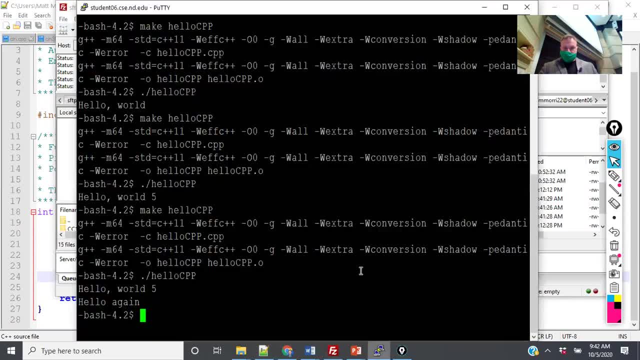 And this will print everything out. And I'll show you everything with a makefile in a bit. 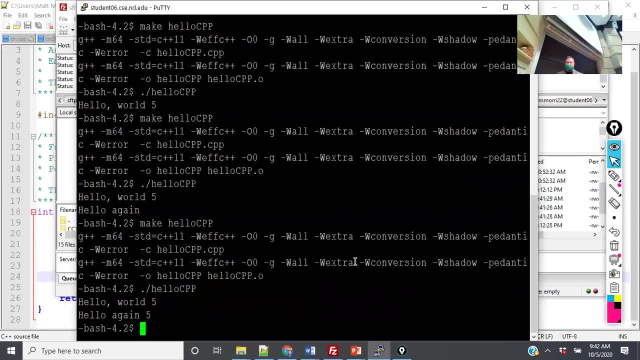 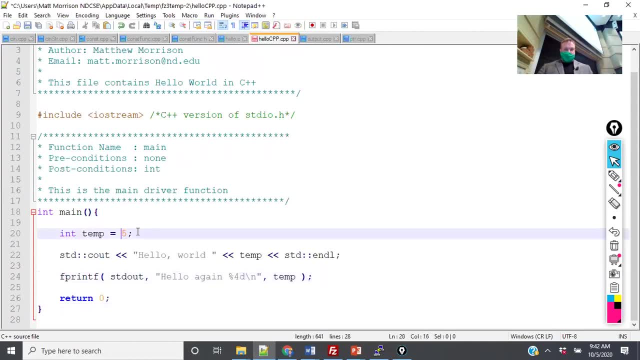 However, let's say I wanted to have a very specific 4, and let's say this is 15. Right? 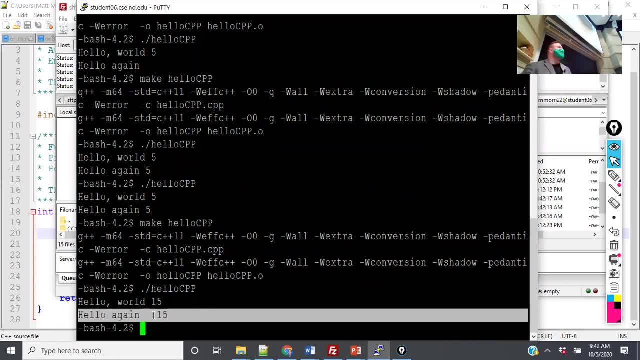 Now, notice how it's created the spaces. So, in C, we can make this much more accurate. 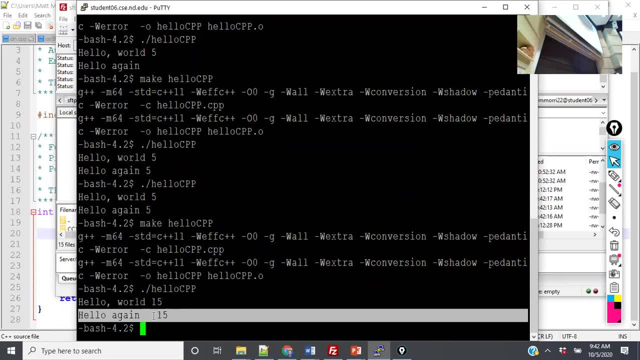 You can do, there are libraries that will allow you to do this in C++, but they're pretty complex. 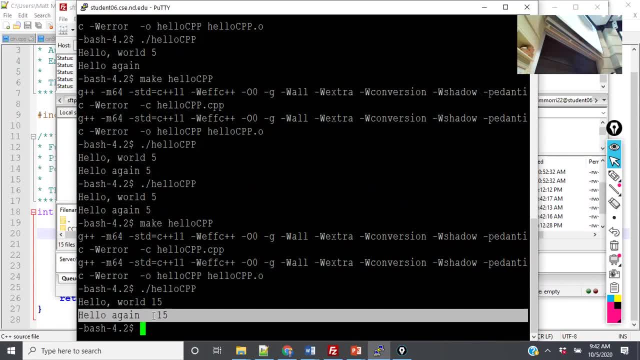 It's called standard, so you can do set precision. But then you have to change it for every single object that you put in. So, one of the reasons why I'm following up on your question in more detail, is because it's a lot easier. . 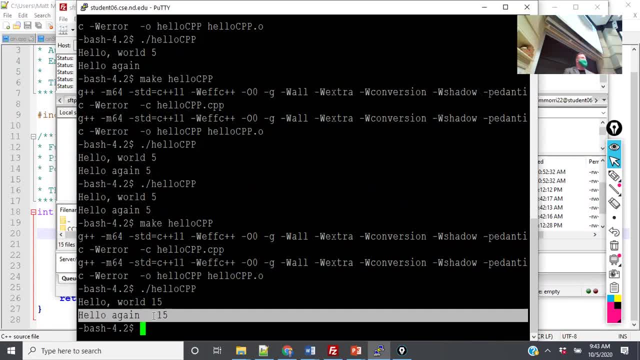 So, one of the reasons why I'm following up on your question in more detail, is because sometimes if you need it to be very precise on the output, some programmers will say, okay, I'm going to default back to the C library in order to get out a very specific set of outputs. 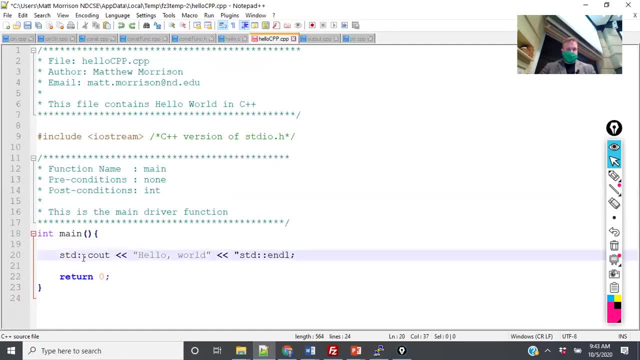 So, let me undo all these changes. . 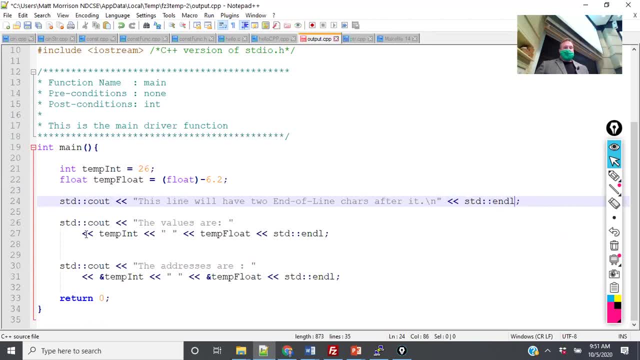 So, this is just several different ways of saying the exact same thing. So, now, here, I'm printing out the values are, and I'm printing out the actual values themselves. 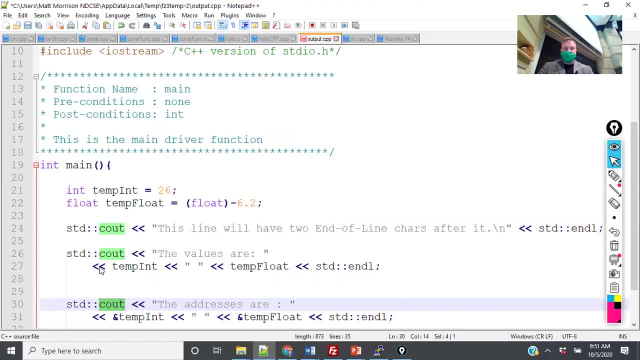 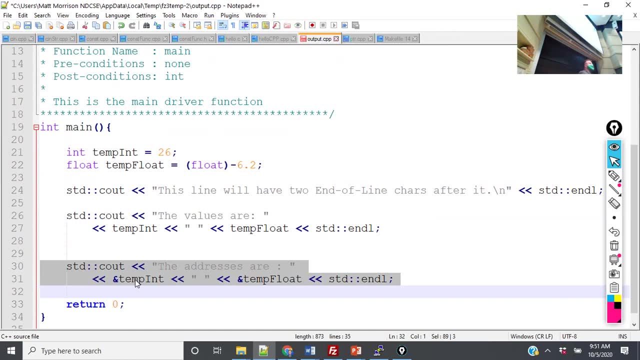 . . . . . . . . No more casting to void pointer, no more %p. 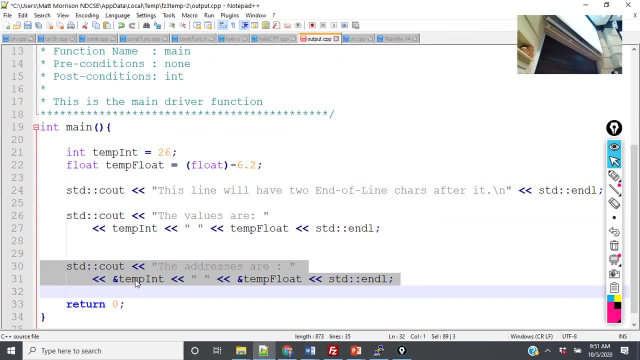 I want the address of the registers, I can just do that and the object-oriented programming language will do the work for me. 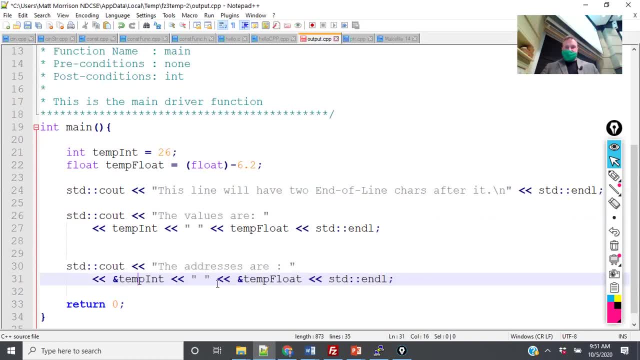 That's a little bit of abstraction. So if I run make output, you see that I have 26 and negative 6.2. 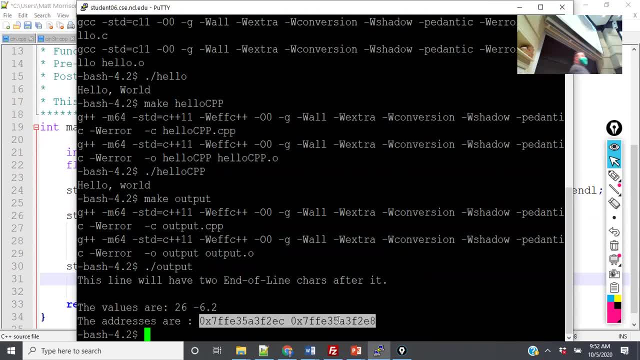 And then I have the addresses of those registers printed out. Yes. Yes. 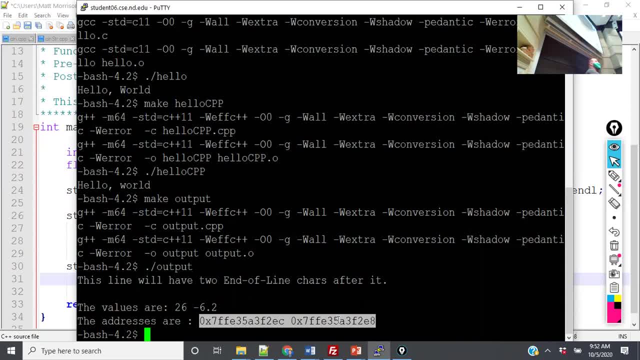 You can also specify the element on the printout where it's deep-referenced by this . Correct. Absolutely. 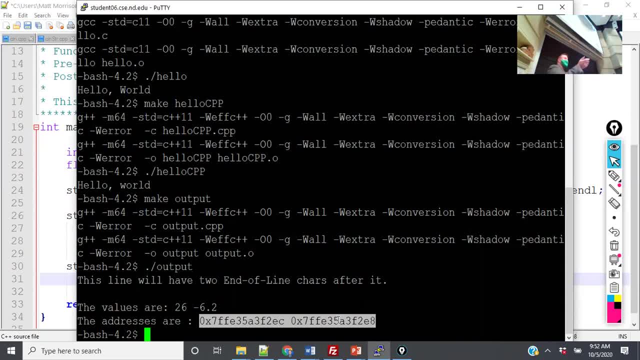 Yeah, so now we can take away that void pointer specification. So it's a little less complicated to code. Object-oriented programming does the work for us. Hey, does anybody have any other questions? 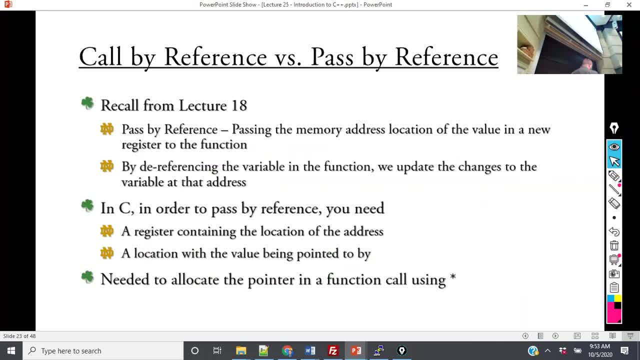 Okay, so next thing, pass by reference. So in C, in order to pass by reference, we had a function that we wanted to pass to. We didn't do one of two things. If we passed an array, so for example, just a character array with strings, or we were passing just a multidimensional array, it passed it by reference by default, right? In C++, it passed it by reference by default. 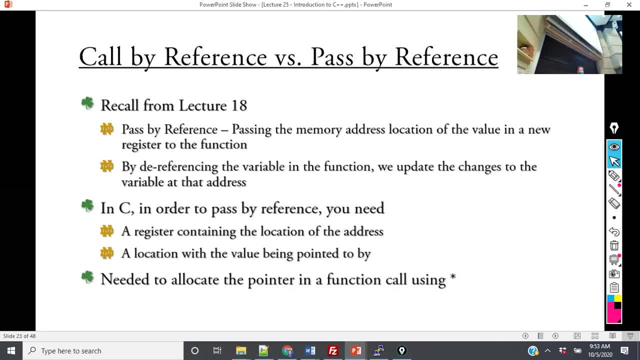 In C++, that's still the same. As we get to C++ arrays, we're gonna see that we have to do it a little differently 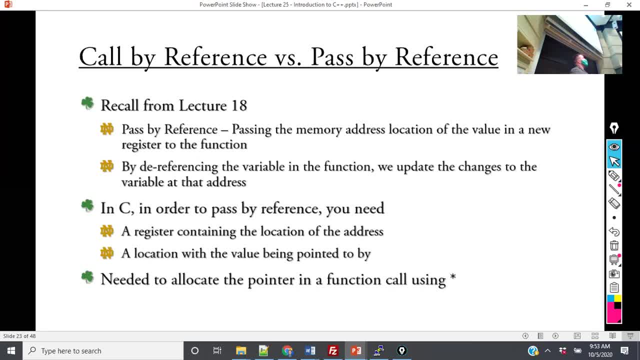 because in the object-oriented programming, it's going to demand that we maintain some data integrity. 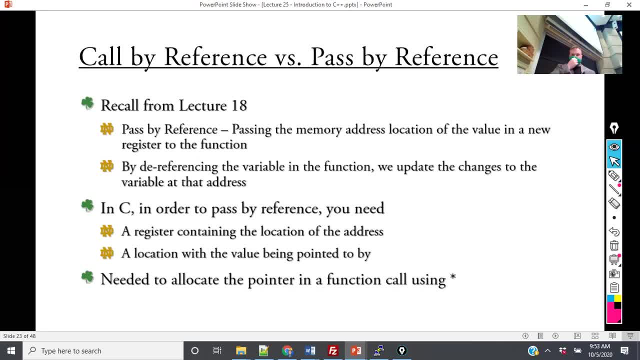 And we're eventually gonna learn about this C++ is this idea of a strongly typed language. 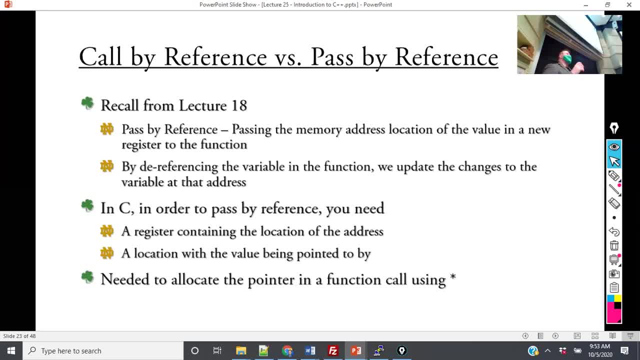 But in short, what we had to do is if we had to pass an integer by reference, what I had to do is I had to do int star, right? 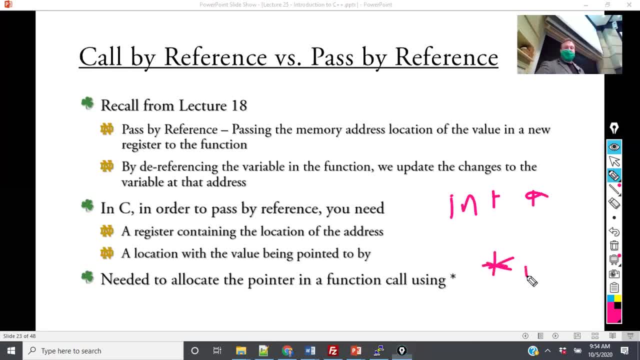 And then if I wanted to get that value, I had to dereference it there, correct? 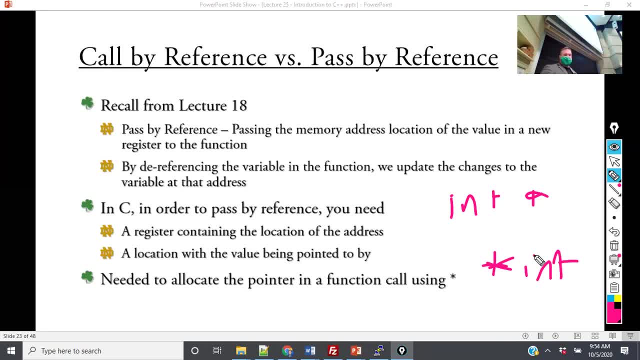 And if I want to save it or grab that information, that's what I had to do. 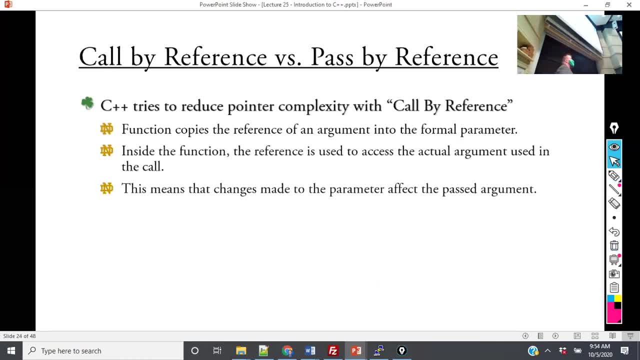 In C++, they have this new concept called call by reference. And the objective of call by reference is to copy the reference of an argument into the formal parameter. And then once you have this done, you can make modifications by writing the code as though it's local. 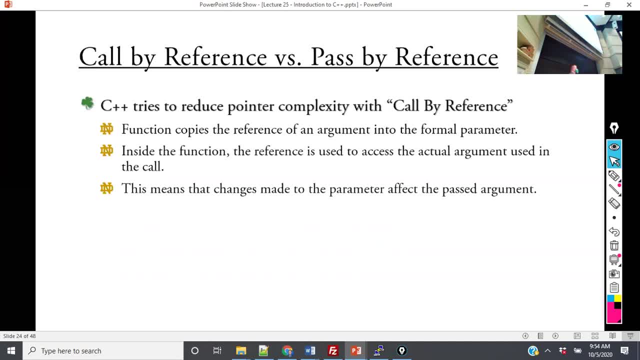 The objective of call by reference is to simplify the process of passing a variable to a function and modifying that unit. 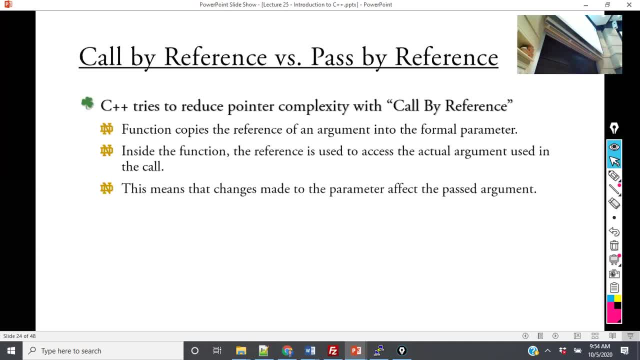 Now, this is another one of those things that if it's a little confusing when I show it to you the first time, do it again. 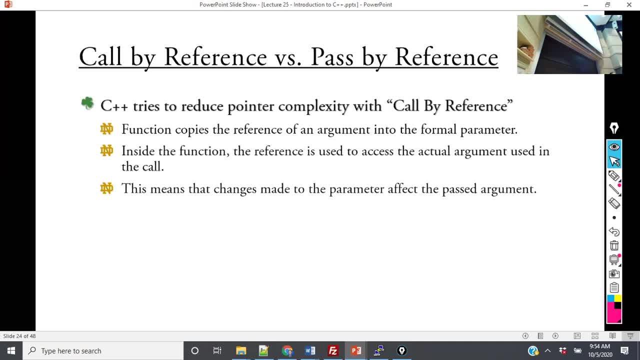 Do not hesitate to raise your hand. Don't get me wrong. Don't hesitate to raise your hand, never. 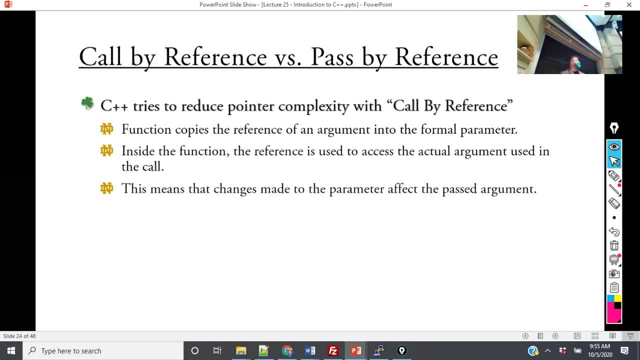 But in this case, if it looks a little confusing and you don't get it the first time, bring the class to a screeching halt. It's perfectly fine. 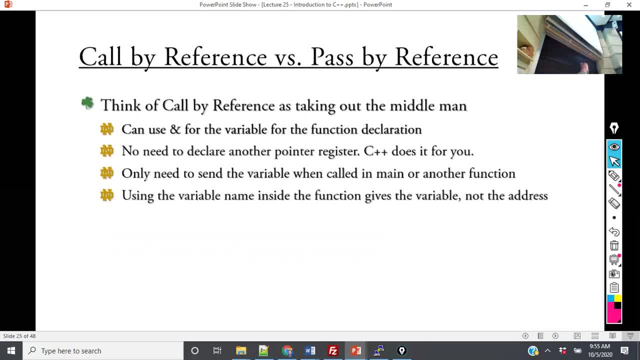 So before I show you call by reference, I want you to think of call by reference as taking out the middleman. What we're going to do is instead of saying int star x, we're going to say int x. And then inside, instead of saying having to dereference it, I can just make the changes without having to do anything to the variable. 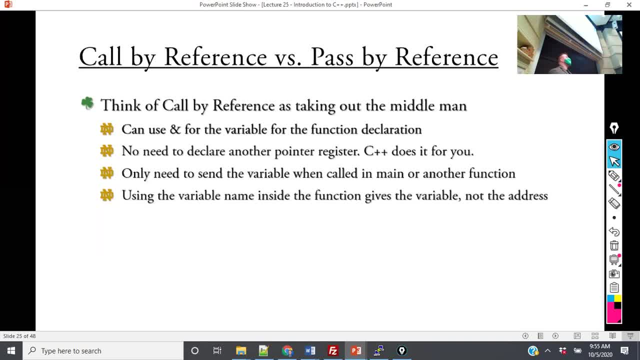 And if I make a change to it, it will automatically make the change. And then when we leave the function scope, that change will be preserved. 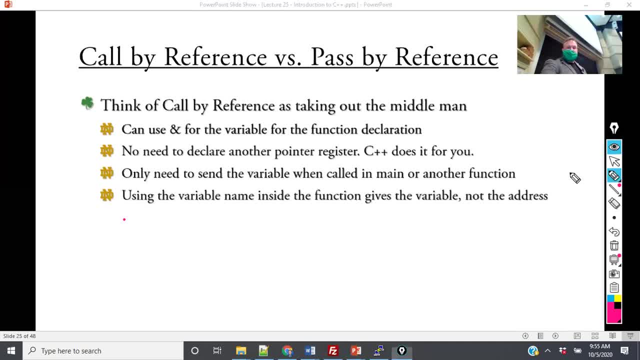 And the benefit, as we'll see in a moment, is that using the variable name in the function gives the variable not the address. So remember, if I, with pass by reference, if I had int star x, and if I did print f, it would give me the address of the variable. 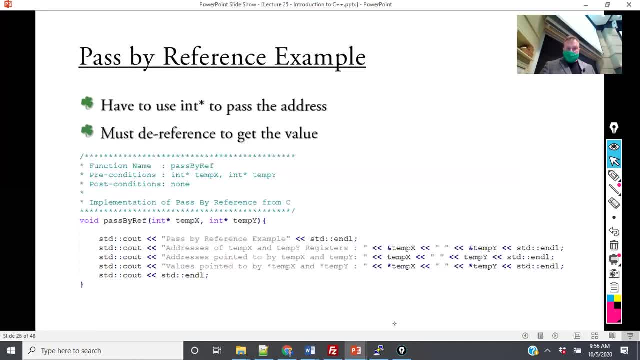 So let me show you an example of what I'm talking about. So first, let me bring up, okay, so it's called pointer.cpp. 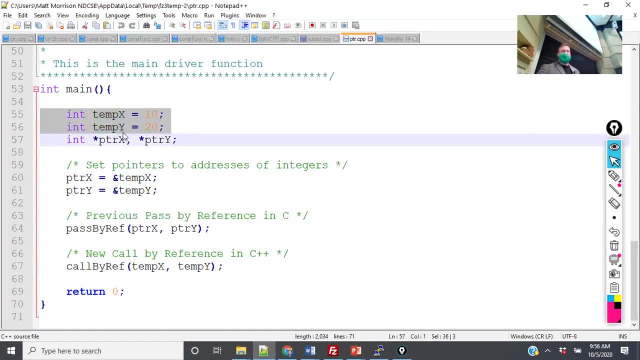 Now, first, let me go to main. And in main, I create two variables, temp x and temp y. And when we did pass by reference in C, I had to create pointers, pointer x and pointer y, right? And to pass by reference, I had to do those pointers. The other way I could have done this is I could have gone 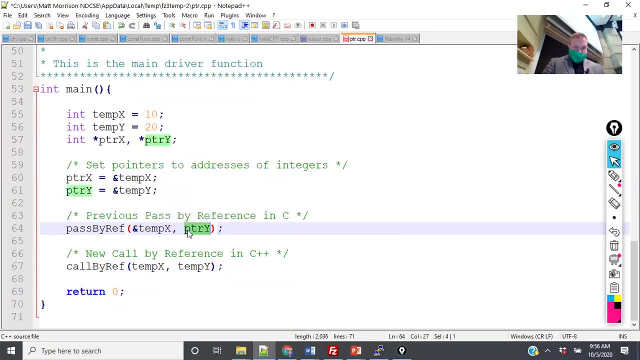 appersand temp x, appersand temp y. 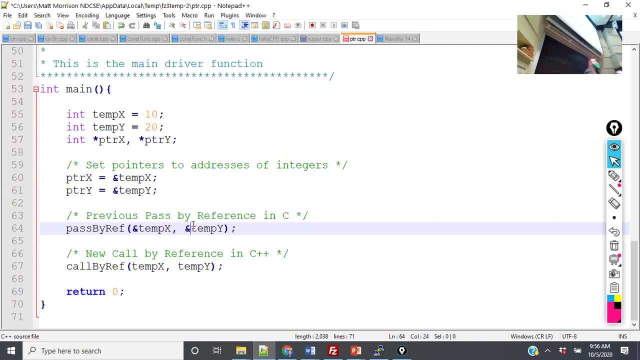 The crucial thing is when I did pass by reference, I had to pass the address of the function, I mean, of the variable. Does that make sense so far? 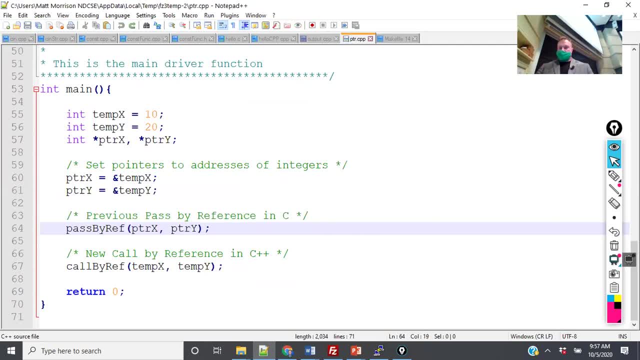 So before I go into call by reference, I'm gonna show you as a review what we were doing in pass by reference. 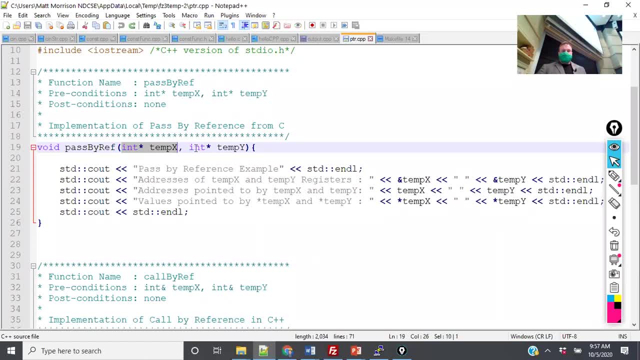 So here I passed pointer to x and a pointer to temp y. 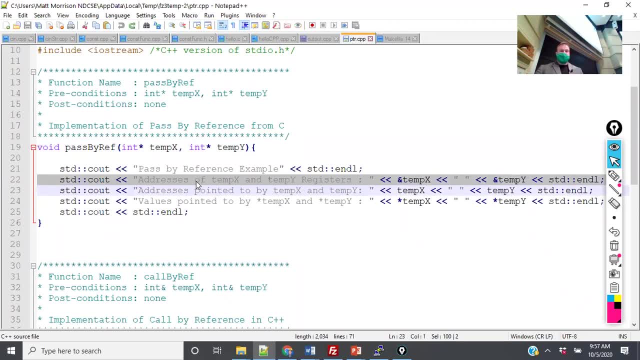 And then I print out the addresses, and that's the address of the function. 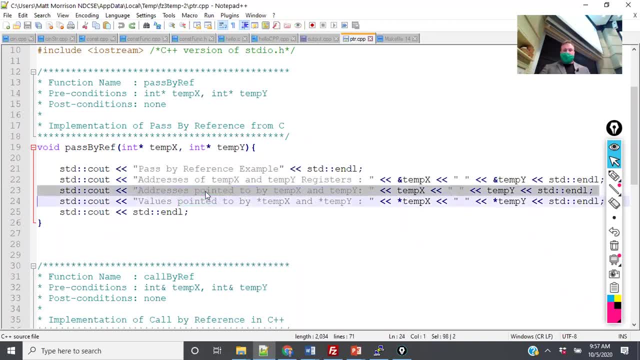 This is the address of the local register. The address is pointed to by temp x and temp y is the value inside that variable, just like before, except in C++, we do not need to pass the void star. 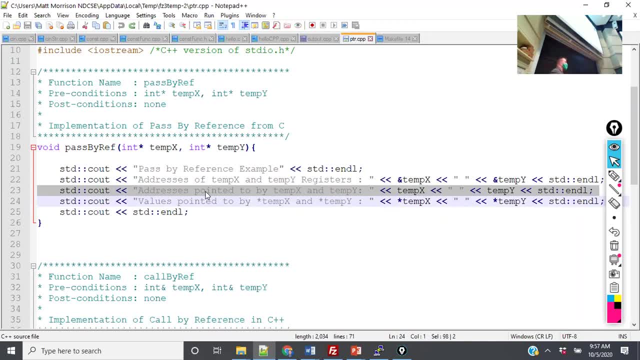 So we're still doing the same thing, going back to the hungry puppy analogy. The address of temp x and address of temp y and pointer is the location where the dog is thinking. The address pointed to by, so Aaron was looking, she was looking at the hand that had food in it, right? That's the temp x and temp y that I currently have highlighted. 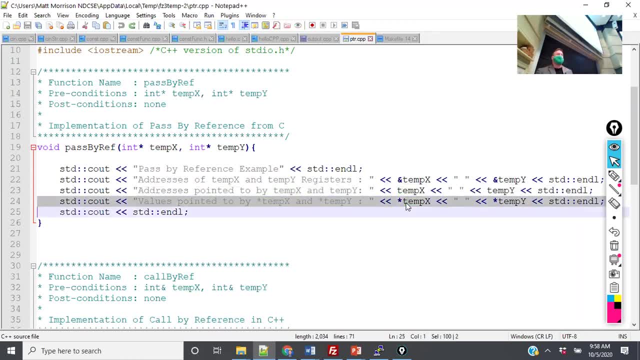 And then dereferencing it, temp star temp x and star temp y is when I reveal the cheese. Everybody remember that? 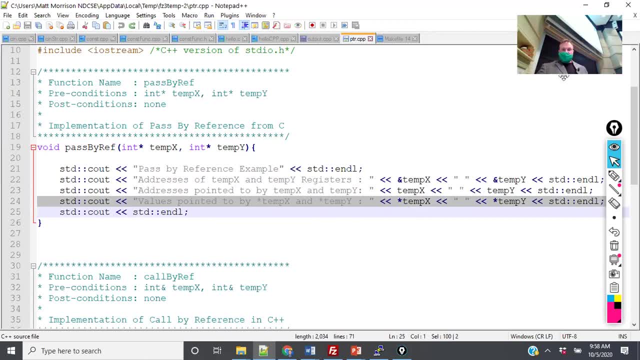 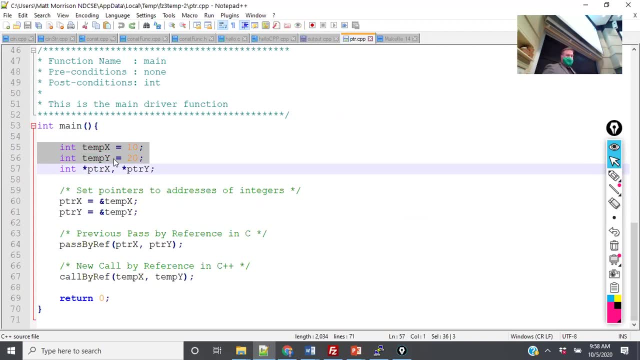 So now let's take a look at this idea of call by reference and see how it's different. In call by reference, you see I have temp x and temp y, and then call by reference, I'm just calling them. I don't have to do any appersand. 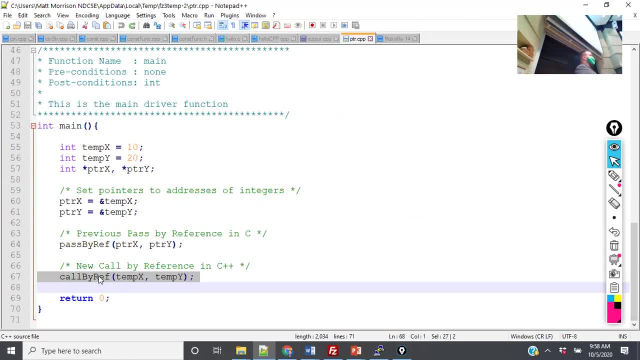 I don't have to allocate any pointers. I don't have to do any of that. Does everybody see that so far? 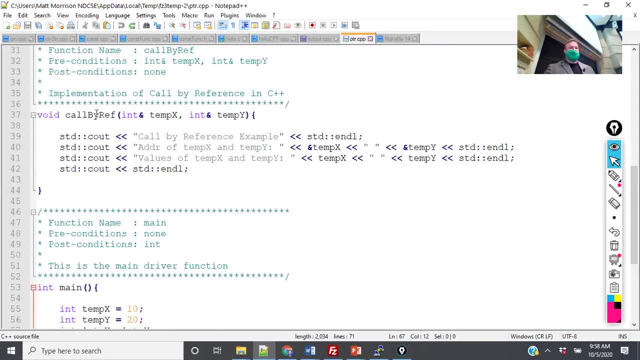 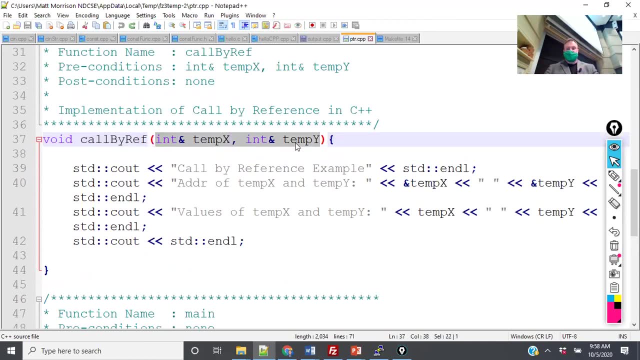 And the reason I'm able to do this with a call by reference in C++ is that in this function, I do int appersand temp x and int appersand temp y. 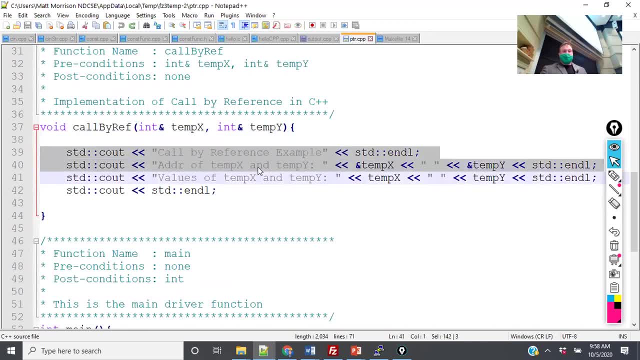 And from there, I have call by reference example, but I wanna say the address of temp x and temp y. And so that's the hand. 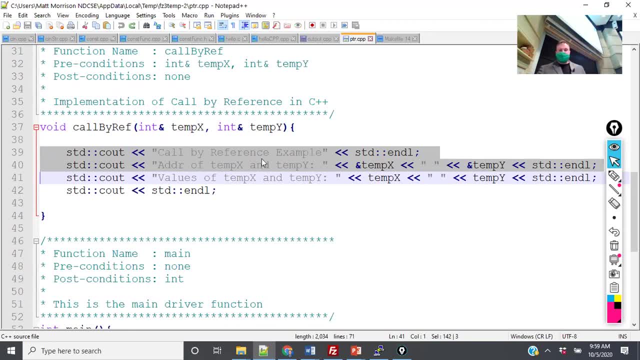 I can say appersand temp x and appersand temp y. And then values, I can just use the values as though it's being written normally in May. 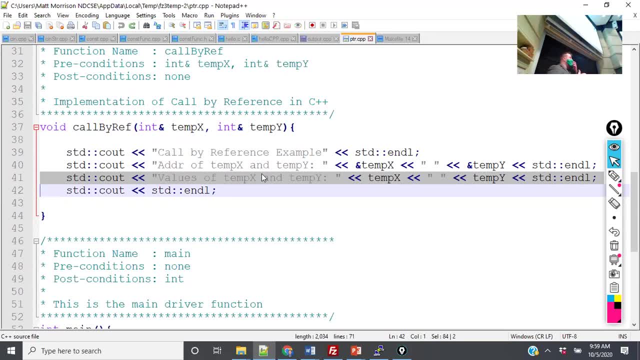 And so what you will see is when I run this, it's gonna do a pass by reference call and a call by reference. This is a call by reference function call. And the thing that you will notice is that the address at this line at 40, where it's saying appersand temp x, because it's being called by reference, this gives me the location. 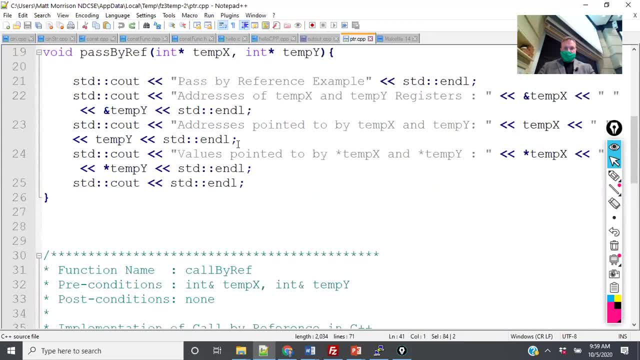 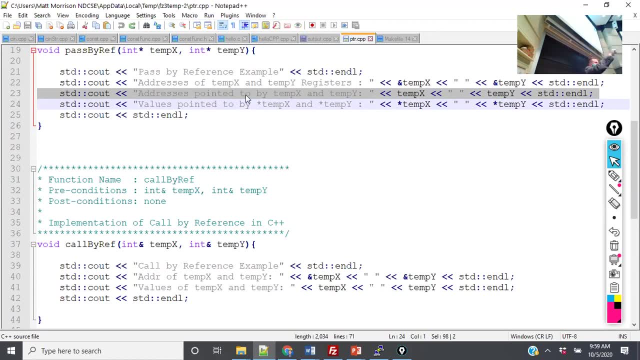 That is the same thing in pass by reference when I say address is pointed to by temp x and temp y. You're gonna see that in the three lines, that in the middle line in pass by reference, it's gonna be the same thing as the addresses of the first line in call by reference. 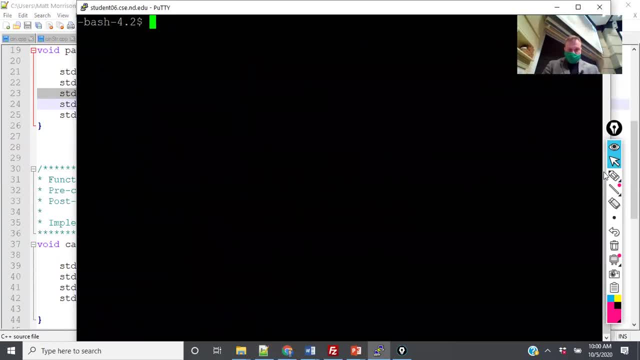 Make pointer, then we're gonna run it and run clear, then pointer itself. 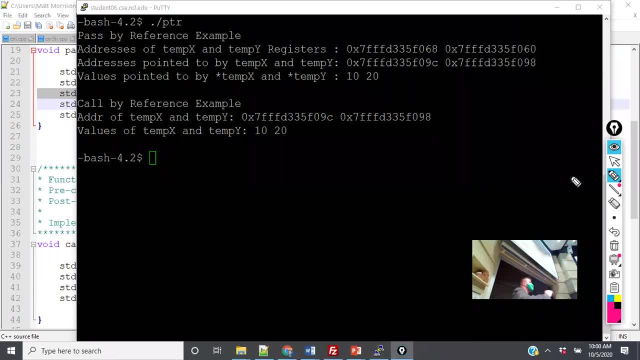 And so to conclude lecture, here's the difference between the procedural pass by reference, where I have to pass these addresses of the registers, right? And then to get the information, I have to go inside the registers and get them from this location. And then these are the dereferenced values. And that's temp x and temp y in pass by reference. 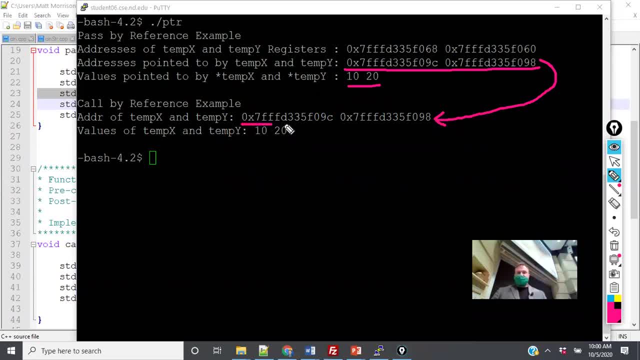 And when I call by reference, when I do that appersand, you'll see that these addresses are the same, which means when I do appersand temp x and appersand temp y, when I call by reference, this means I am getting the address where the variables, are located, which means that I've cut out the middle man. 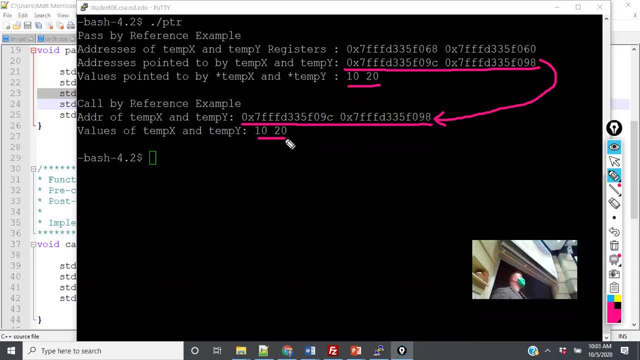 And then when I just say temp x and temp y, I just get the values themselves. 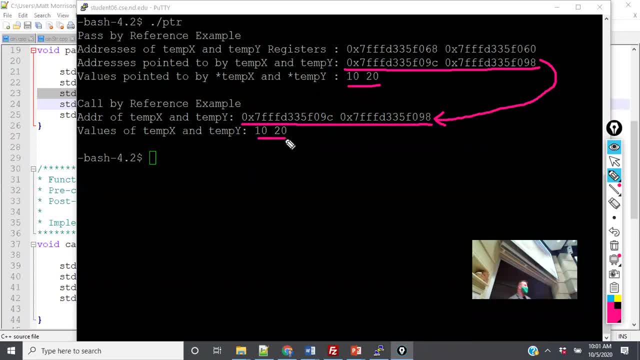 So the objective of call by reference is to treat variables that are passed by reference as objects in order to abstract coding complexity from the program. Does everybody see that? Okay. 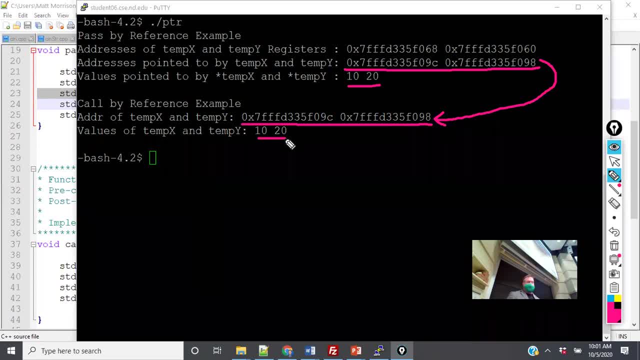 So this is where we'll conclude for today. And then we're going to pick up on more C++ on Wednesday.